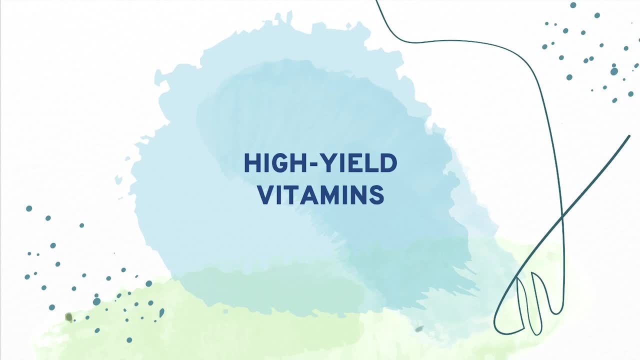 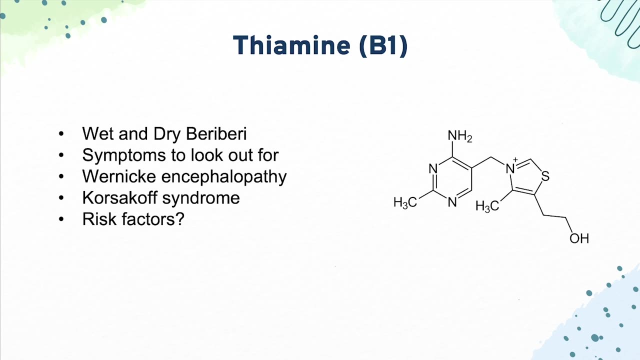 essentially at least a couple of questions about vitamins on your exam. So with that let's get started. The first vitamin to look out for is thiamine, also called B1. So one of the ways this is commonly tested in the clinical context is through the avenue of beriberi. There's two kinds. 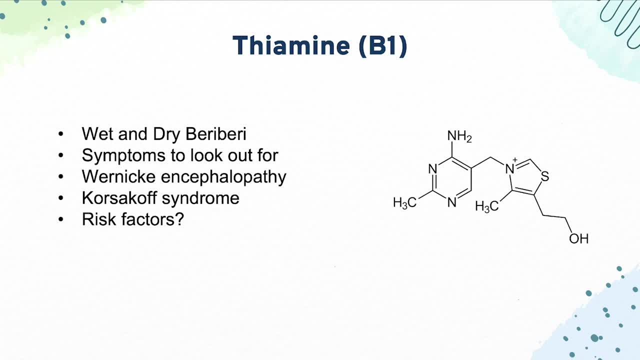 of beriberi, wet and dry. So wet beriberi is essentially the same as dry beriberi, except wet beriberi has the addition of something called high output heart failure. Essentially, the heart becomes dilated and cardiac output is increased. That's on top of dry beriberi, which typically involves damage to nerves and 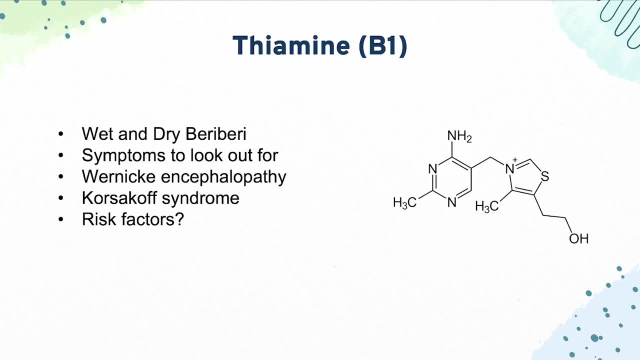 muscle atrophy around the body. So if you see someone who maybe is malnourished and they're having muscle wasting and nerve issues, that is one of the things to definitely consider. Then we get to Wernicke encephalopathy. Wernicke is characterized by a couple of common symptoms. 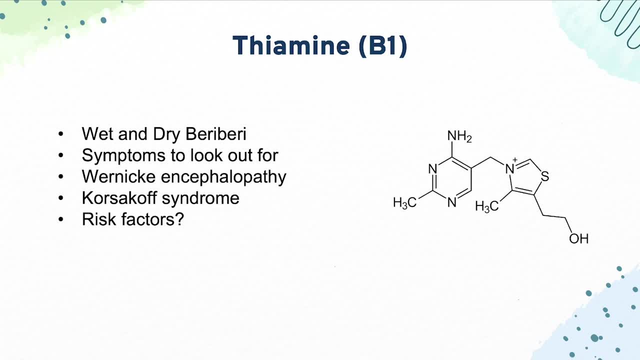 which you can memorize via the mnemonic can-o-beer, Also because one of the risk factors for thiamine deficiency is alcoholism. So, can-o-beer, The C stands for confusion, the A for ataxia, the N for 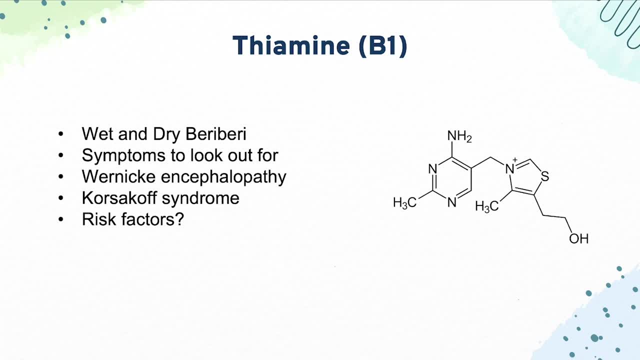 colugia and beer just reminds you that alcoholism is a risk factor. So if you see someone who presents to the ED, a lot of times they'll say that the eyes aren't able to look in one consistent direction as a way of tipping you off to the nystagmus. Maybe they smell of alcohol. One of 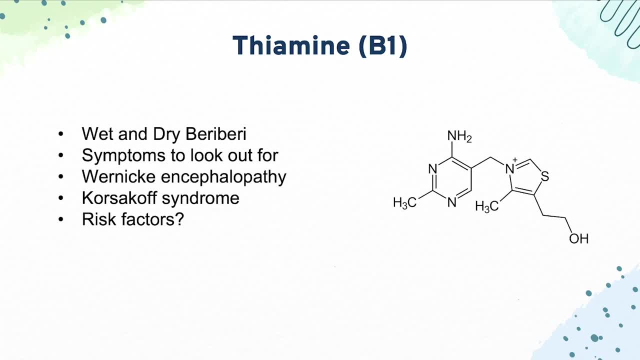 the things to consider definitely is Wernicke encephalopathy. Korsakoff syndrome is similar, but what marks Korsakoff syndrome is something that is not a common symptom. So if you're called confabulation, Confabulation is essentially when people forget certain. 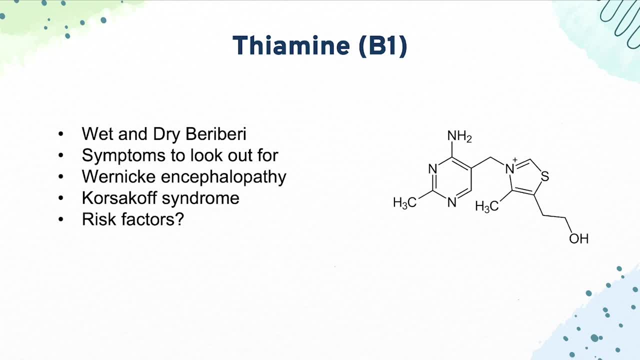 periods of recent time in their lives and they fill it in with details that didn't actually happen. So, for instance, you could have a person who comes to the ED and when asked how they got there, they were apparently brought on a magic carpet. Of course they weren't brought on. 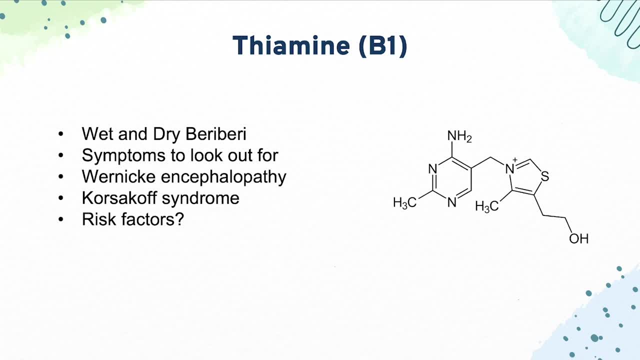 a magic carpet, but that is their way of filling in the details that they don't know. And they're not trying to fake anything. They're just trying to fill in the details because they themselves don't know. When you combine Wernicke-Korsakoff syndrome- one of the things that the USMLE loves- 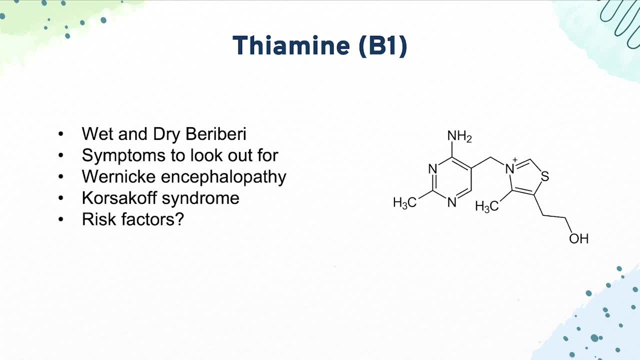 to test is what exact part of the brain, which anatomical structure, is damaged. And that is the medial dorsal nucleus of the brain. And that is the medial dorsal nucleus of the brain, And that is the medial dorsal nucleus of the thalamus or the mammillary bodies. And with Wernicke-Korsakoff. 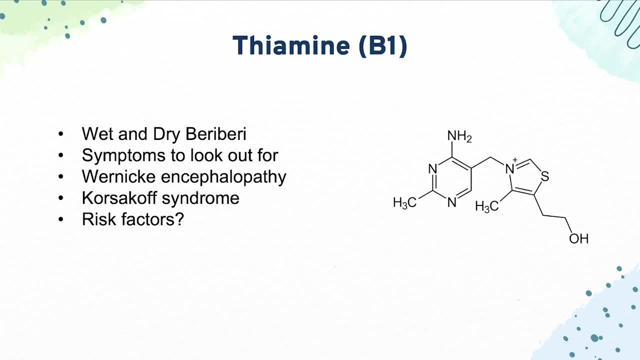 syndrome you have all of the symptoms of Wernicke and the confabulation of Korsakoff. So the can-o-beer symptoms of Wernicke and then the confabulation of Korsakoff, And those are essentially the high yield points for thiamine or B1. 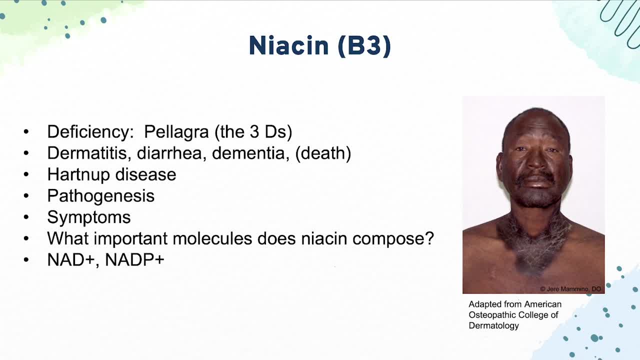 Next we get to niacin. So a deficiency of niacin, which is also a very high yield thing to know for the step exams for all of them is something called pellagra or the three Ds. Those three Ds are dermatitis. 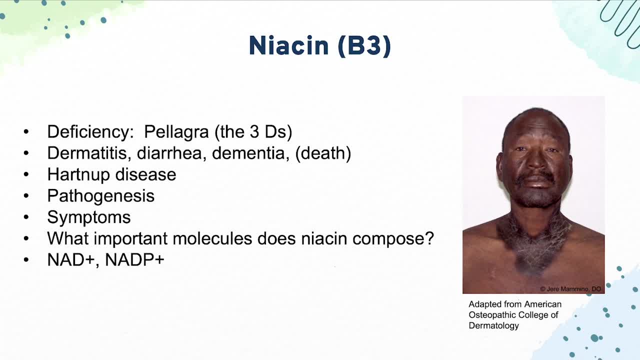 diarrhea, dementia and some people add a fourth D which is death. The dermatitis typically presents like in the picture on the right here, with that necklace sort of appearing distribution Of skin irritation, And that is a very commonly tested image on these step exams. 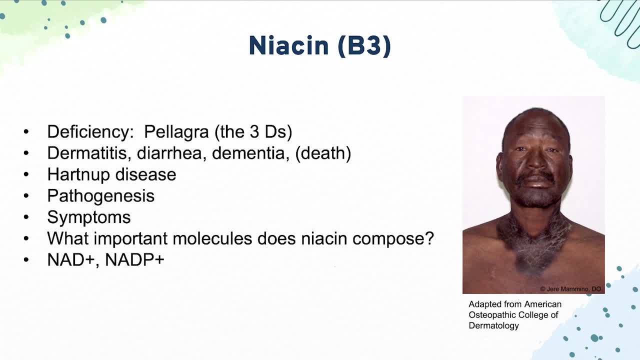 One of the ways that a niacin deficiency can manifest is with something called heart and up disease, So for this we have to go back into a little bit of biochemistry. So with heart and up disease you lack the transporters in the proximal renal system, And so you have to go back into the 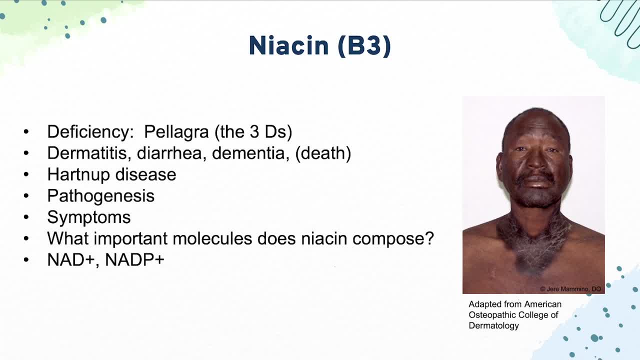 proximal tubules And with that you can't reabsorb the neutral amino acids. One of the neutral amino acids is tryptophan, which, coincidentally, tryptophan, is a main component of niacin. So in heart and up disease you can't reabsorb tryptophan in the kidney and you urinate. 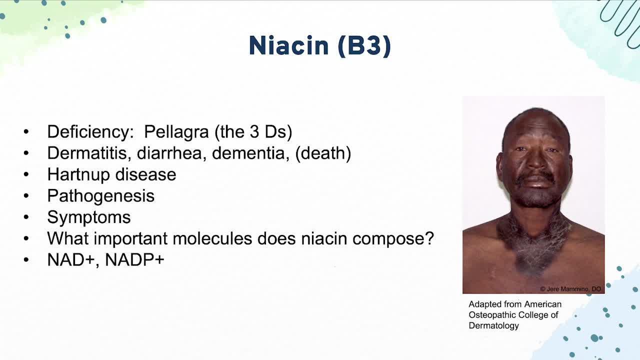 it out. That can lead to a niacin deficiency or eventually pellagra, Because you simply don't have the ingredients needed to make the niacin. That's a very commonly tested pathology on the step exams. The symptoms, as I was saying, mainly the things to know are the dermatitis, diarrhea, 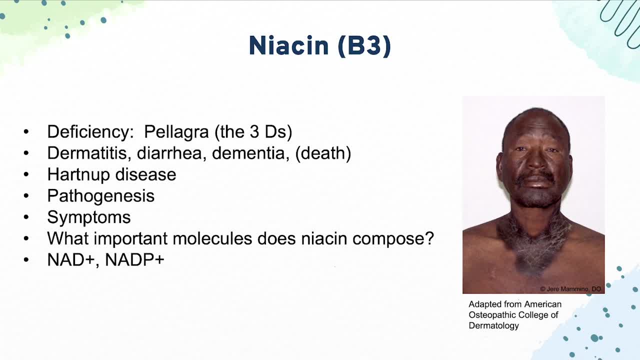 and dementia, Potentially death, becomes that severe. Again, it's important to know that tryptophan is a main constituent of niacin, But it's also important to know what niacin itself is needed. So niacin is needed to act as one of the main ingredients in the molecules. 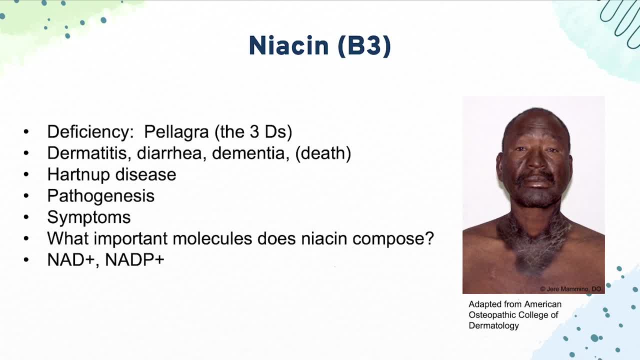 NAD plus and NADP plus. Both of those play important roles in energy production, in both glycolysis and the TCA cycle. They're involved in redox reactions, in which NAD plus and NADP plus are converted to NADH and NADPH respectively, And those eventually can fuel the niacin. 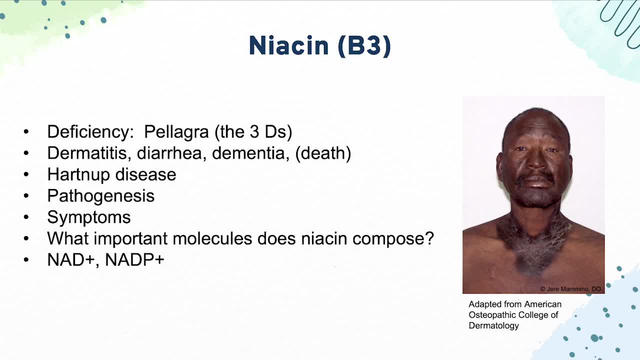 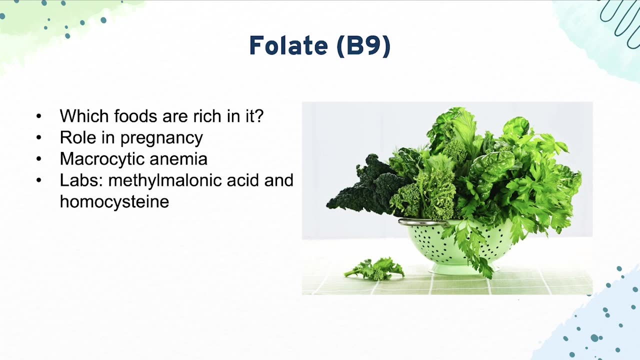 On to the electron transport chain. So it's clear that niacin plays some pretty important roles and thus is a very testable vitamin for the step exams. I'm going to skip a bit ahead to the next high yield vitamin, which is folate B9.. 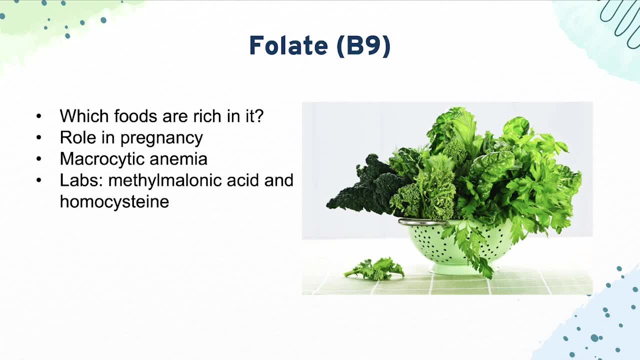 One of the things to know is that folate comes primarily from leafy green vegetables, things like spinach, kale, stuff like that. It's also important to know that it plays a really big role in pregnancy. The folate is needed to promote neural tube closure. 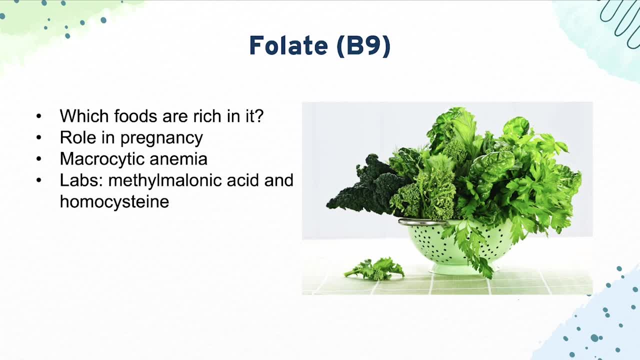 in embryos and fetuses. So if you don't have folate, the baby's going to have neural tube defects. That's why in pregnancy you have to usually supplement with folate. Also, with a folate deficiency you can get a macrocytic anemia, which 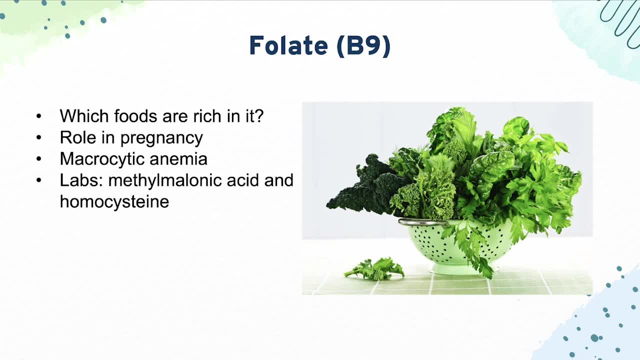 as a little bit. you are going to have over six lobes in your red blood cells and they're going to have an MCV of over 100.. For the labs, you're going to want to check the methylmalonic acid and the homocysteine levels. So with this case, the methylmalonic acid is going to be normal. 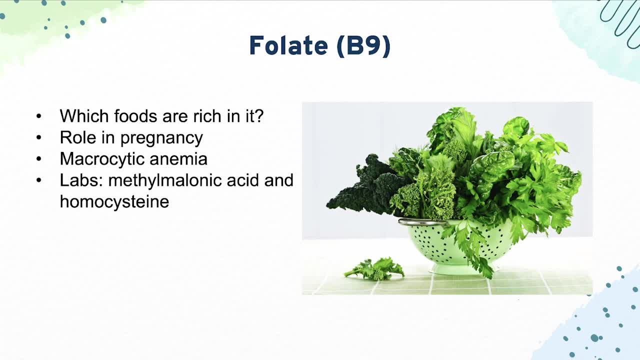 but the homocysteine levels are going to be elevated. That's going to be in contrast to one of the other vitamin deficiencies we're going to see in a bit. One other thing to know for folate is just generally about the functions that it does in. 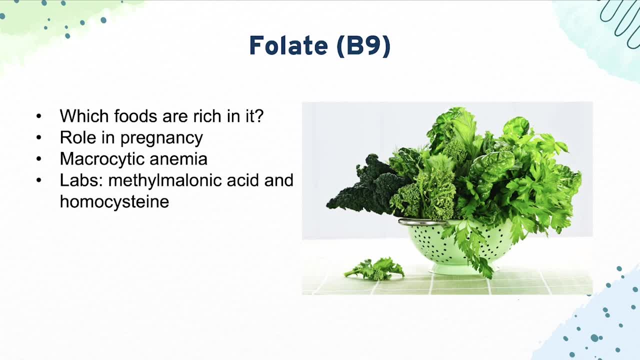 the body. So folate composes primarily, among other things, tetrahydrofolate, which plays a important role in methylation reactions, So that involves moving one carbon from one molecule to another. It also plays a big role in making nitrogenous bases, So things like deoxyribonucleotides and 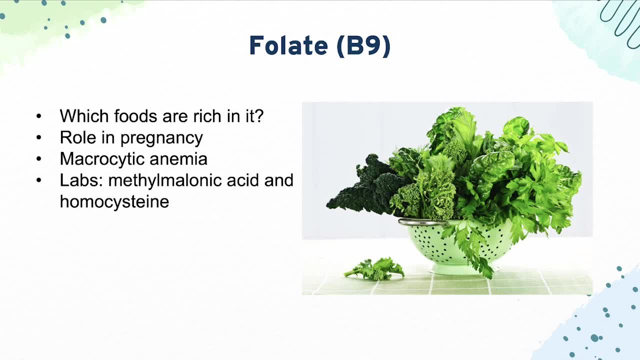 ribonucleotides. One of the last things that they like to test is where folate is absorbed in the gut, and that primarily is the jejunum. So the main takeaways for this is that folate is involved in methylation reactions, plays a role in the neural tube for pregnancy. 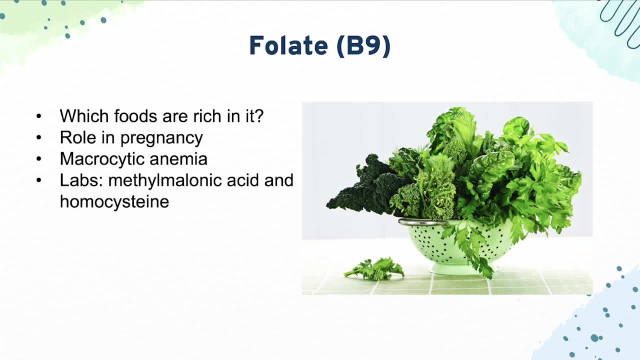 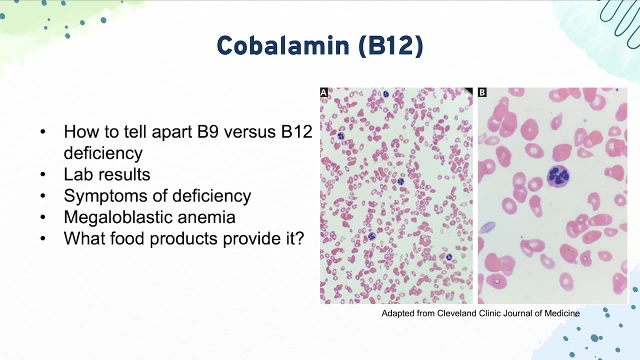 and a defect or deficiency rather, can lead to a macrocytic anemia. Next we come to cobalamin or a vitamin B12. So a B9 and B12 deficiency can look pretty similar, And that's because if you have a deficiency in both, that can lead to the megaloblastic anemia. 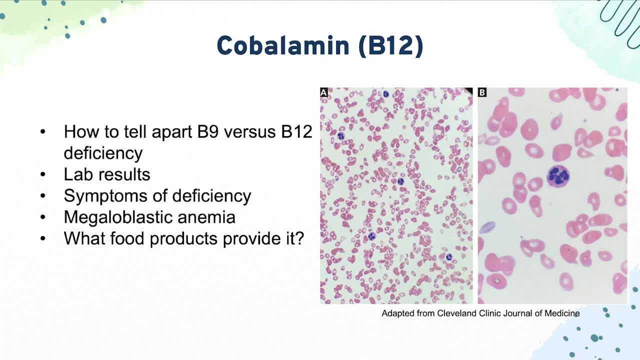 Like you see on the screen, there's that red blood cell with over six lobes present. Still, there are certain ways to tell it apart. So, with a B12 deficiency, unlike a B9 deficiency, one of the things that you're going to have is something called subacute combined degeneration. 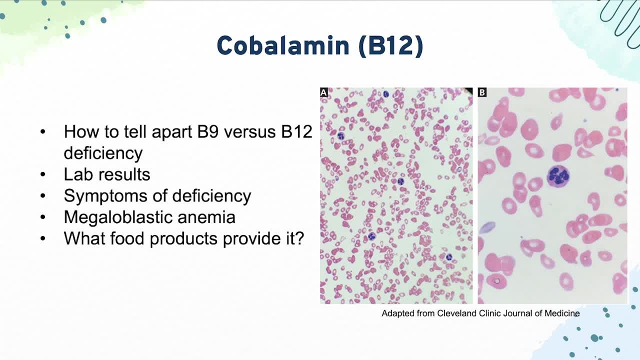 That's going to generally manifest in a lot of neuropathic symptoms. So what you're going to have is weakness. You're going to have sort of tingling and numbness in your hands and feet. You're going to be a bit clumsier than normal. That's what people describe. 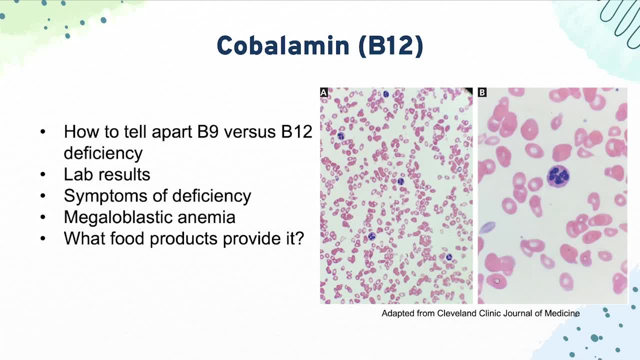 It's a general loss of proprioception in the extremities. So if you have that along with the elevated MCV, that would suggest a B12 deficiency For the lab results. so, unlike before, with a B9 deficiency when you have the elevated homocysteine levels, 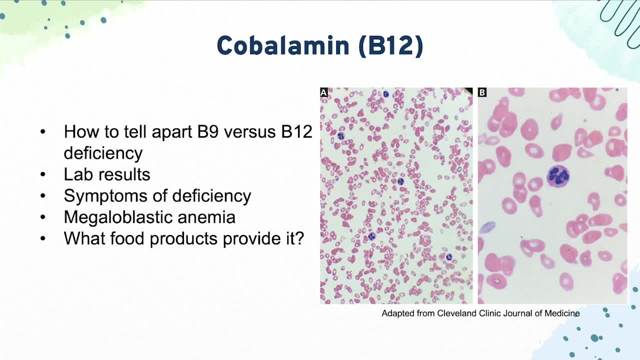 but the normal methylmalonic acid levels. here you would have an elevation, an elevation of both. So that would be an elevation of both the homocysteine and the methylmalonic acid. And that's just because these vitamins are involved in different enzymes and processing different substrates. 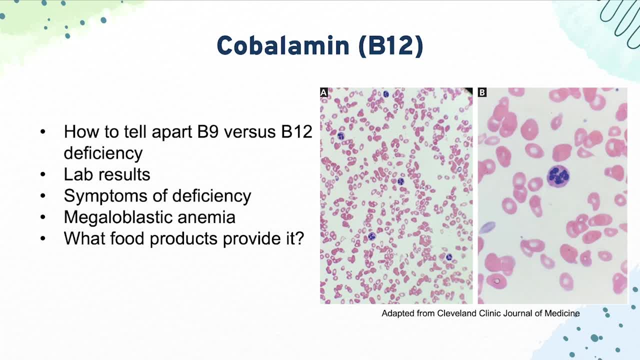 So overall things can accumulate on the back end. One of the other high yield facts that's tested for cobalamin or B12 is what food products provide it, So that primarily is going to be animal products, any kind of meat, things like that. 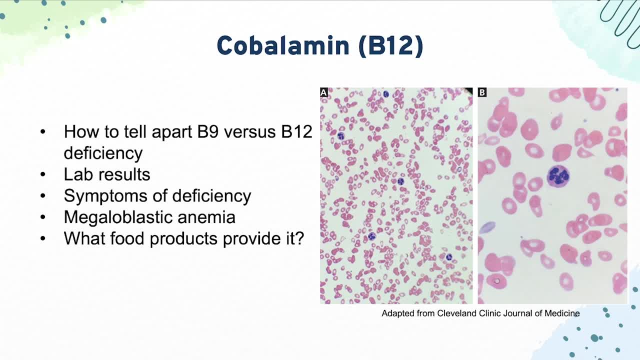 And where it's stored is in the liver, And B12 can be stored in the liver for years, So it's typically a little bit rare to see someone who has a B12 deficiency due to a lack of meat in their diet. Eventually, if after years and years of not consuming animal products, it's possible, sure. 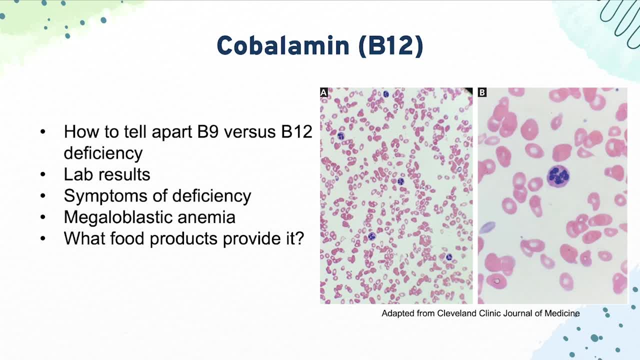 But the USMLE typically doesn't do that. They typically won't test it in that fashion With a B12 deficiency. one of the things they typically will test is pernicious anemia, where you get antibodies that kind of destroy the ability of B12 to work and be absorbed. 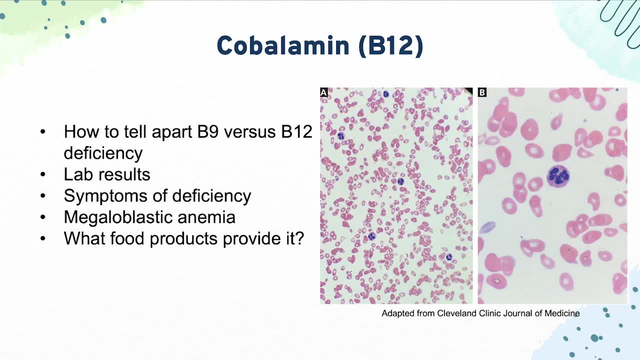 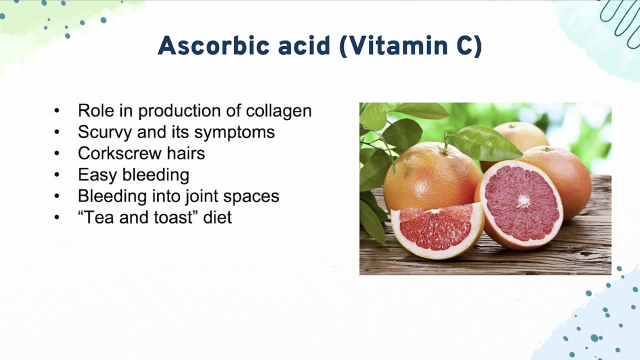 One of the ways that they will test the deficiency of B12 is through something called pernicious anemia, where you get antibodies against something called intrinsic factor and then you have less B12 absorption. Our next vitamin is vitamin C, also called ascorbic acid. 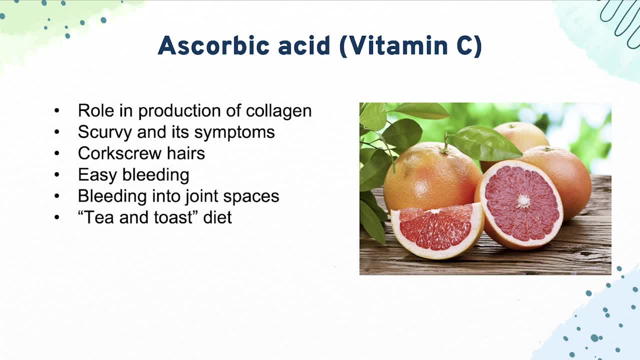 So vitamin C plays a pretty important role in the production of collagen And with that it does hydroxylation, So it attaches an OH group to proline and lysine residues on collagen And with that it can stabilize the triple helix of the molecule. 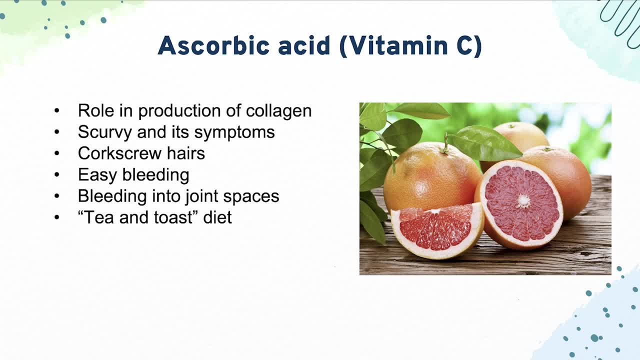 When you don't have a B12 deficiency, you have that kind of stabilization that can lead to a bunch of different symptoms and sequelae, which collectively could be known as scurvy. So one of the things you can have is corkscrew hairs. 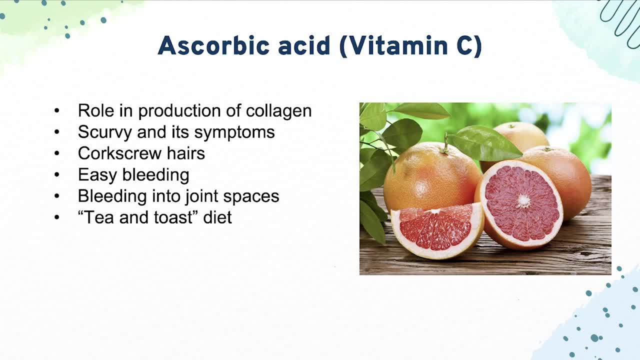 and that's because you don't have the stabilization of the structural components in the hair. One of the next things is easy bleeding and bleeding into joint spaces, And one of the ways that the USMLE test writers like to trick students is to make them think that patients have hemophilia rather than vitamin C. 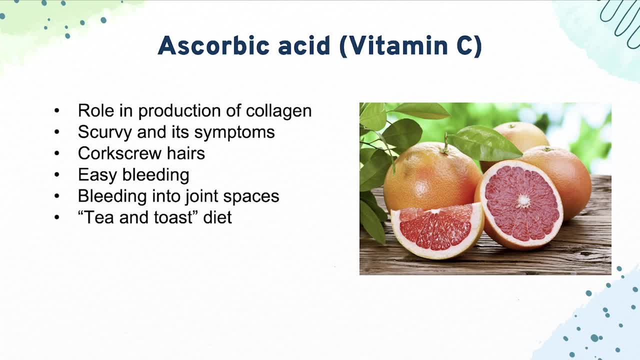 leading to the bleeding into joint spaces. The bleeding into joint spaces is typical of both a vitamin C deficiency and hemophilia, But the difference is. for vitamin C deficiency, it's because you don't have the strength of the vessels required, because you have a deficiency in collagen. 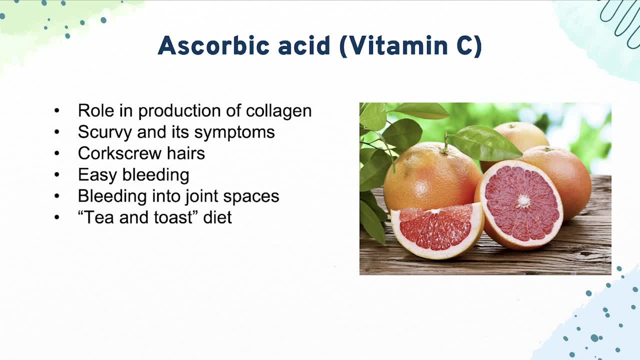 and then that leads to the bleeding. Otherwise, something called the tea and toast diet leads to vitamin C. That's because vitamin C is typically found, among other things, in citrus fruits, And if patients, especially elderly patients, are only having tea and toast, 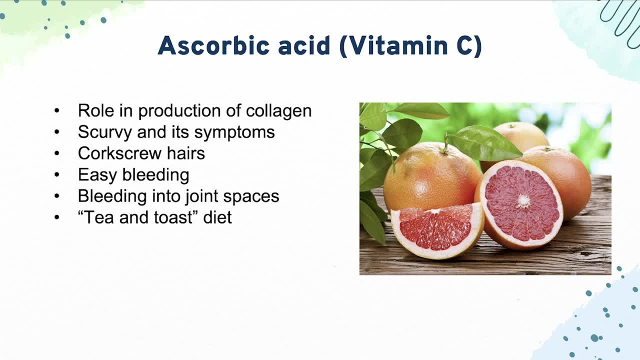 as it's usually called, they can develop a vitamin C deficiency. And if they come to the office with those corkscrew hairs with easy bleeding, petechia bleeding into joint spaces, all those things might clue you into a deficiency of that vitamin. 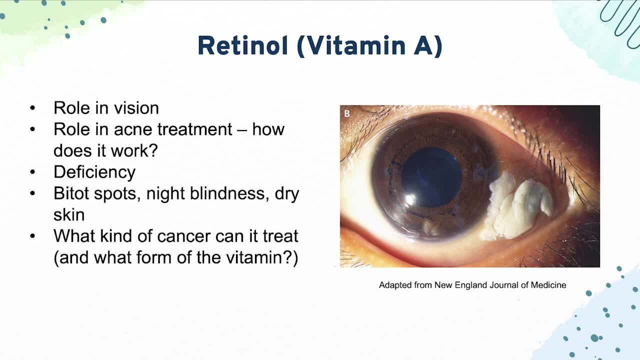 Next we come to retinol, or vitamin A. So vitamin A plays a really important role In vision, And that's because the opsins, which are photoreceptor proteins in the eye, are based. they're composed of vitamin A in part. 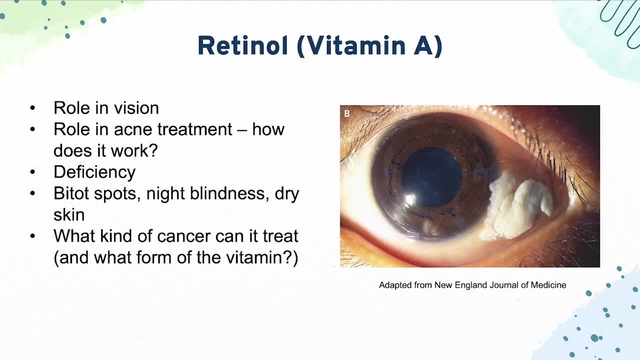 So you need vitamin A to see. One of the other ways that vitamin A is important is that it can be used in acne treatment, And the primary way that the vitamin A works is it promotes re-epithelialization and turnover of keratinocytes. 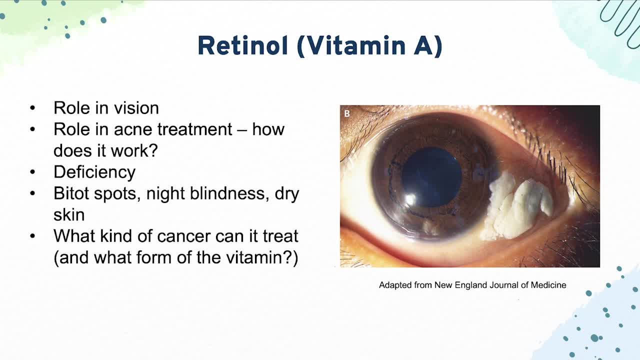 which can help clear the skin of acne. One of the commonly tested enzyme deficiencies on the USMLE is a vitamin A deficiency. So with that you get a whole range of symptoms. So you get things called BTO spots because vitamin A, among other things. 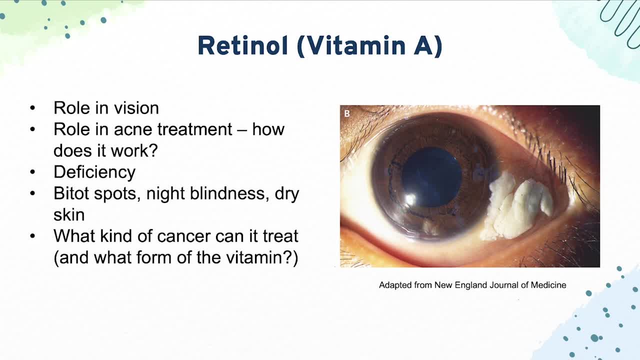 is needed for normal differentiation of keratinocytes. If you don't have vitamin A, you can get things like metaplasia and dysplasia. So the BTO spots, like you can see in the image on the right on the eye. 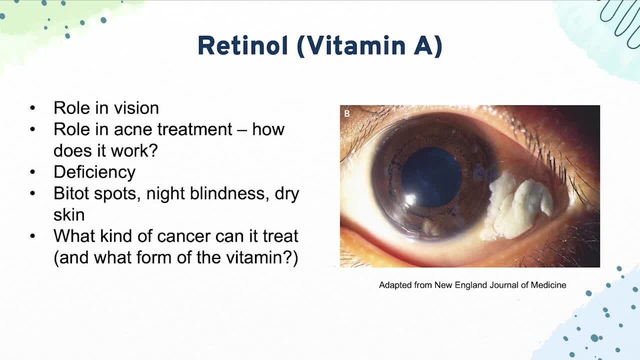 can develop. You can also develop night blindness, which means you just simply can't see at night, and also dry and scaly skin. Interestingly, vitamin A can be used to treat a certain kind of hematologic cancer, And they love testing them. 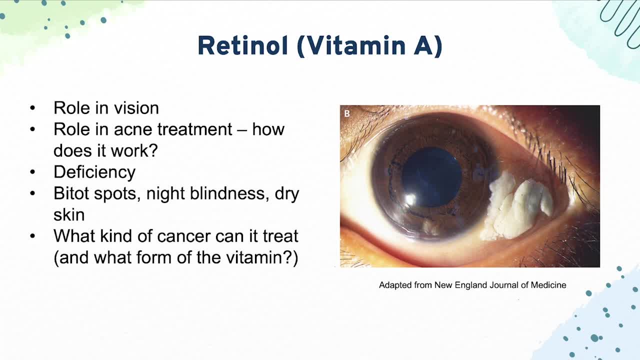 And they love testing this, And that cancer is called APML, That's, acute promyelocytic leukemia. For that you would need a form of vitamin A called ATRA, which is all trans-retinoic acid, Of course. 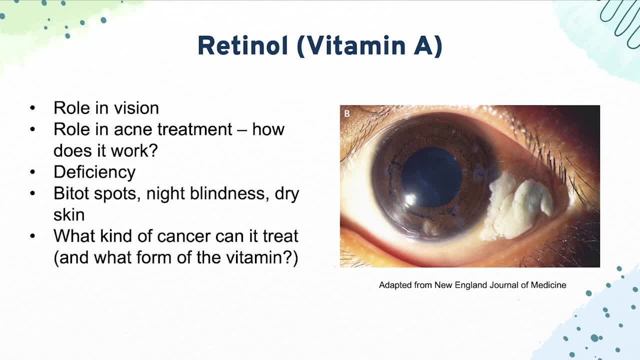 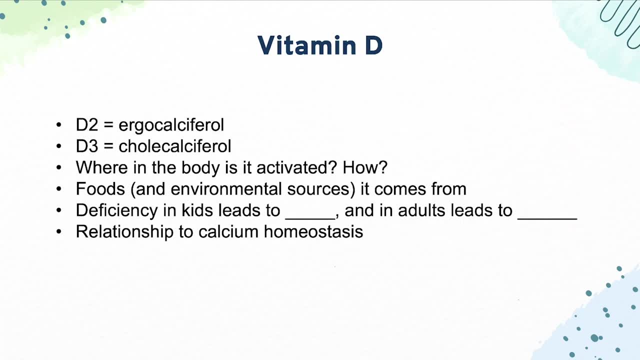 vitamin A is retinol and it can come in different flavors and forms. So if you have all trans-retinoic acid, you would use that to treat the APML. Next we come to vitamin D. So vitamin D is interesting. 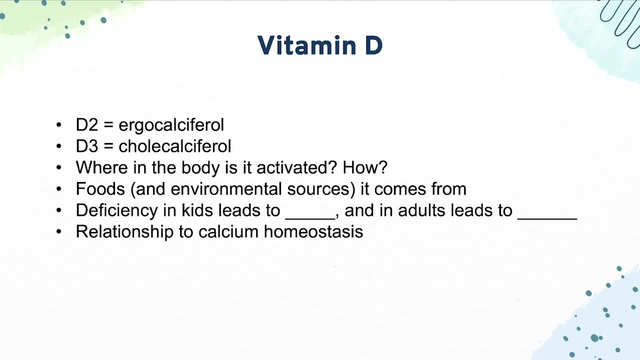 It plays a lot of important roles in the body, especially when it comes to calcium homeostasis. There's different forms of the vitamin, So there's D2, which is ergocalciferol, and D3, which is cholecalciferol. 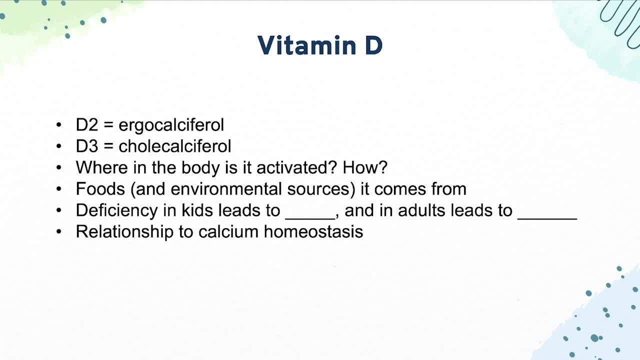 The important thing to know about vitamin D is that it's usually not absorbed in an activated form. It has to be activated. It has to be activated in the kidneys via hydroxylation, So you get 125-OH-D3, or that is the activated form of vitamin D. 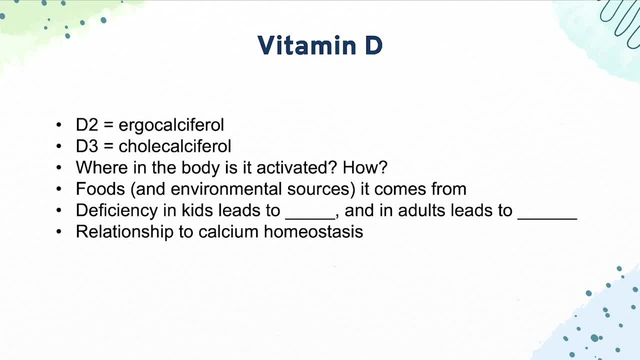 where it can exert its effects on calcium homeostasis. Typical foods that it comes from are things like dairy products, And in the environment it often comes from sunlight, Or rather, it promotes the reaction that is used to activate vitamin D. A deficiency of vitamin D in kids can lead to rickets. 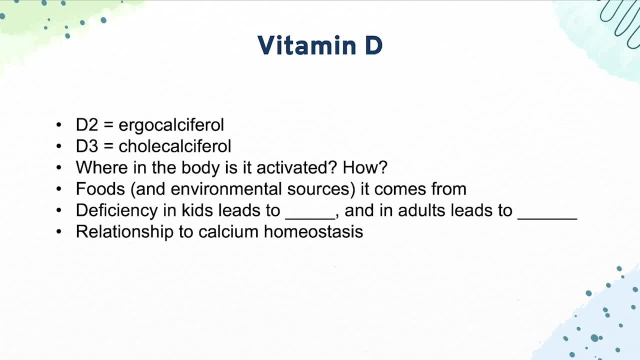 And in adults it can lead to osteomalacia. And then, of course, as I was saying, it has a pretty important role in calcium homeostasis. So I want to spend some more time on that, because they do test that a lot. 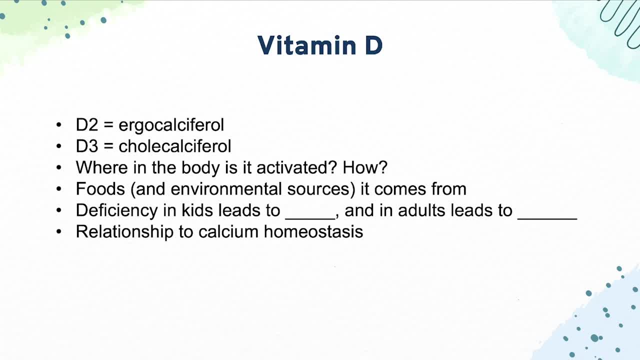 If you have elevated parathyroid hormone, decreased calcium or decreased phosphate, all of these things will lead to an increase in the activation of vitamin D, that 125-OH form, because vitamin D is going to want to increase the absorption of calcium. 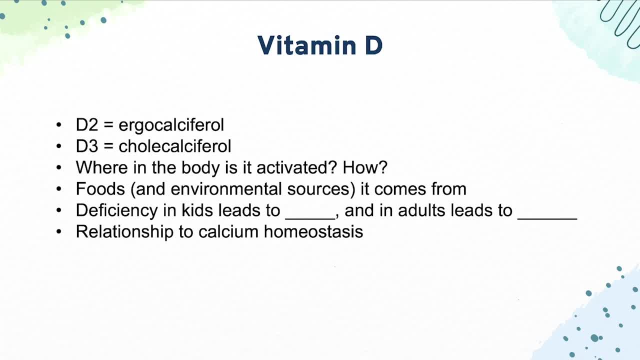 So things like an elevated PTH, which would suggest that you don't have enough calcium in the body, are going to want to increase vitamin D. Also, when you have the activated form of vitamin D, that 125-OH2D3 product- 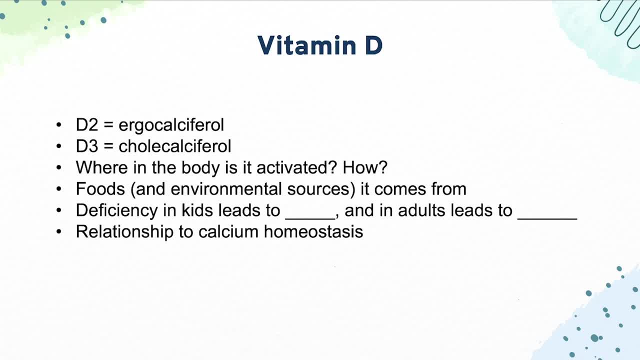 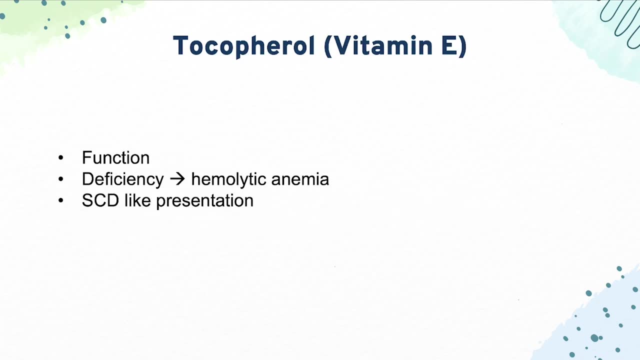 that's going to feed back more upstream and it's going to stop the production of further vitamin D, because or else you could be at risk for having too much calcium. So those are the high yield points of vitamin D to know. Next, we have tocopherol, or vitamin E. 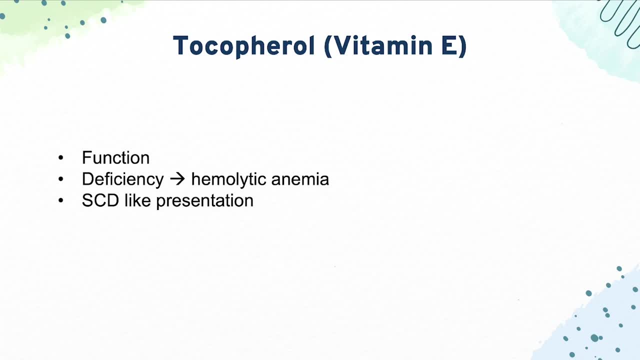 This may not be the highest yield vitamin, but they do test it occasionally And I would want you guys to get it if it came up. So it functions primarily as an antioxidant, taking care of free radicals in the body, things like that. 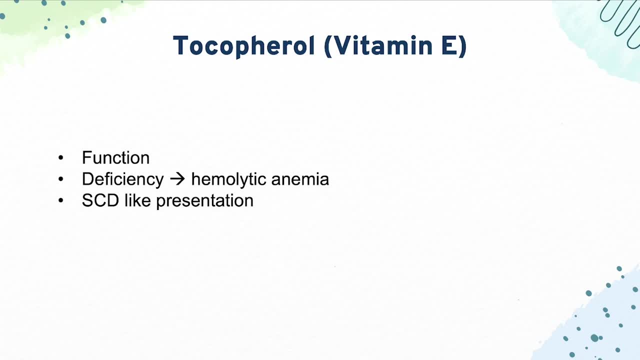 A deficiency of vitamin E is going to lead to hemolytic anemia. So you would be able to see on a blood smear the red blood cells that are burst, but also to differentiate it from other conditions. you would have a hemolytic anemia. 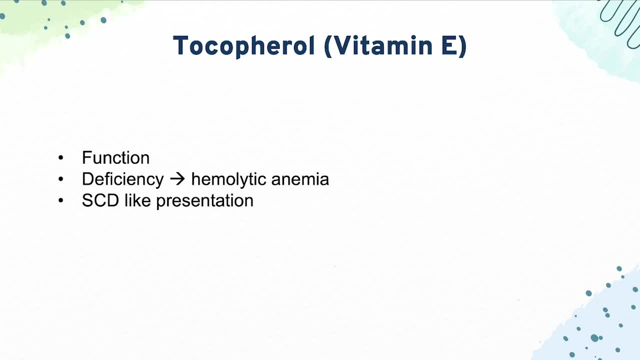 alongside that subacute combined degeneration like presentation. So if you have a patient who looks like they have a B12 deficiency, they have the numbness and tingling in their hands and feet, but they also have a hemolytic anemia. 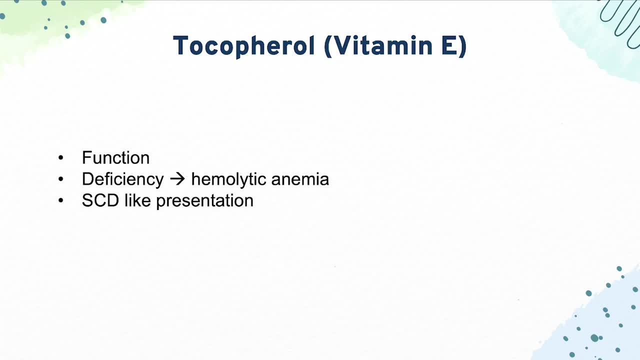 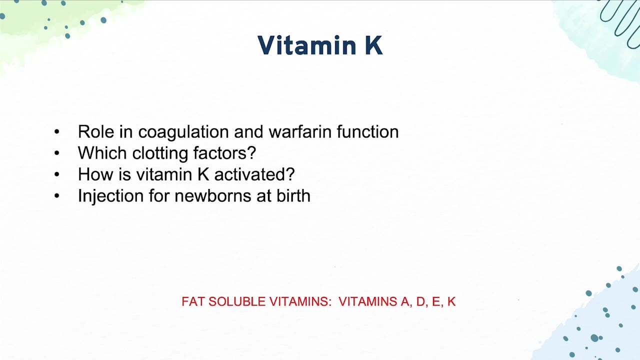 So, for instance, they don't have an MCV of something like 120.. That would make you want to think of a vitamin E deficiency instead of a B12 deficiency. Our last vitamin is vitamin K, So vitamin K plays a really important role. 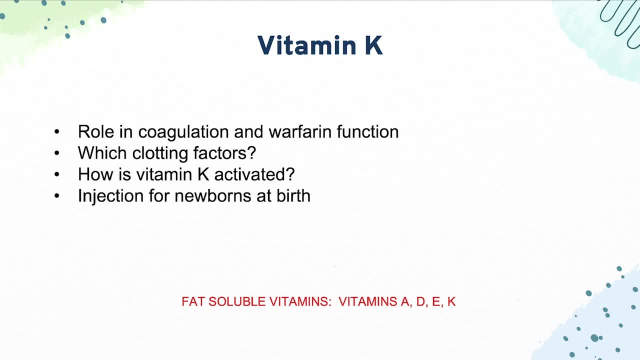 in a lot of clotting functions and also it has interaction with a lot of different commonly used drugs like warfarin. So vitamin K is activated by an enzyme called epoxide reductase. This is the enzyme that warfarin inhibits. 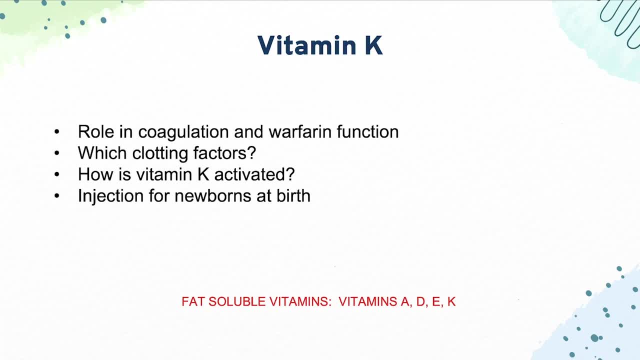 So if you block the epoxide reductase by warfarin, you don't have vitamin K and you reduce the clotting functions of the blood, which is how warfarin works. Vitamin K is needed for modification of glutamate residues. 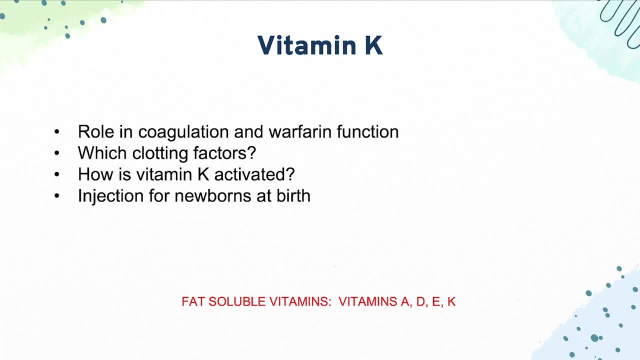 most importantly through gamma carboxylation. It's also important to know which factors vitamin K inhibits. So it inhibits factors 2,, 7,, 9, and 10.. So that's both the intrinsic and extrinsic coagulation pathways. 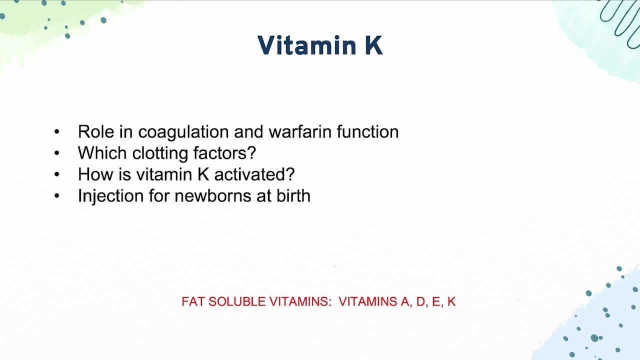 One of the other things to know for vitamin K is that newborns need an injection of it. So vitamin K is in part synthesized by intestinal flora, And when newborns are born they don't have the intestinal flora that can make that vitamin K. 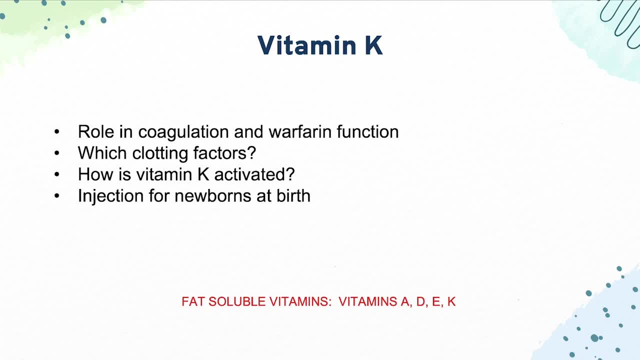 So if a baby is born, for instance, at home, and isn't in the hospital to get the injection of vitamin K, they could potentially bleed out later on because they don't have the vitamin that helps with clotting in the blood. So newborns need a vitamin K injection. 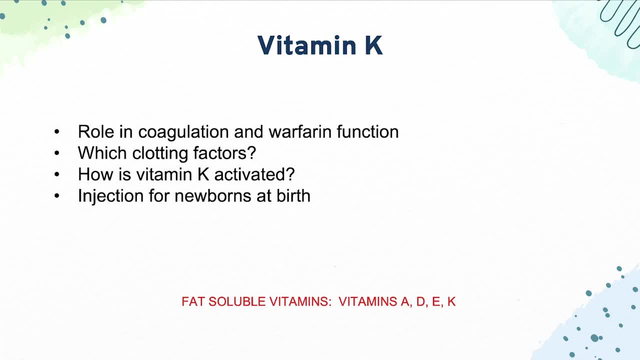 One of the other high yield things to know just overall is that the fat soluble vitamins are vitamins A, D, E and K. All those are absorbed in similar manners as opposed to the water soluble vitamins, And they do test that as well. 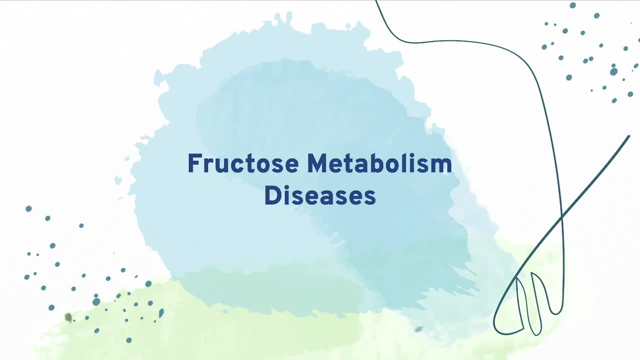 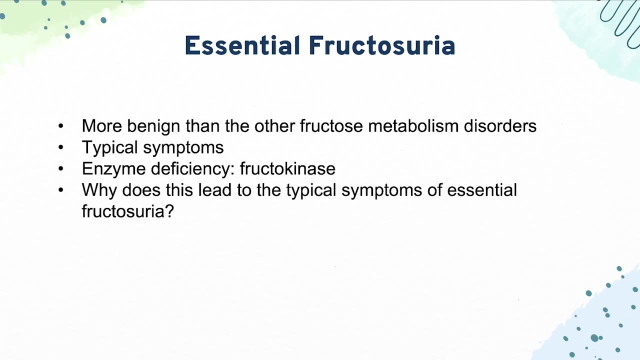 Our next topic is the fructose metabolism disorders. So first we come to essential fructose area. So this one, as opposed to hereditary fructose intolerance, is a bit milder. The typical symptoms are a result of the disease process itself. 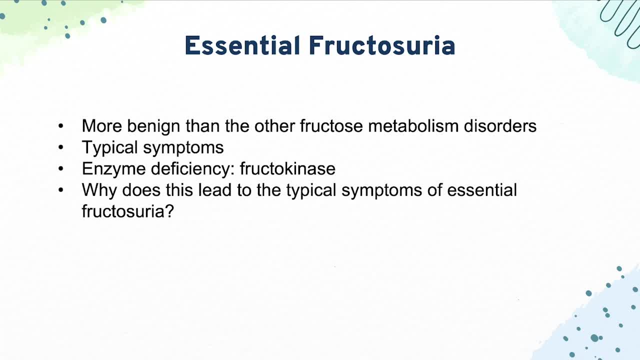 So with this condition you have a defect of fructokinase. So with that you don't have fructose being phosphorylated and then trapping it inside the cells. So fructose can go inside and outside of cells as it wishes. That leads to fructose in the urine. 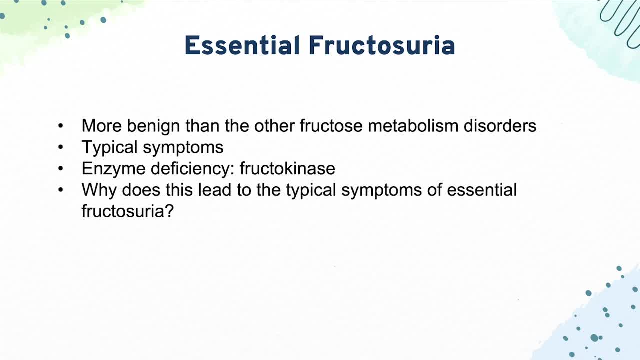 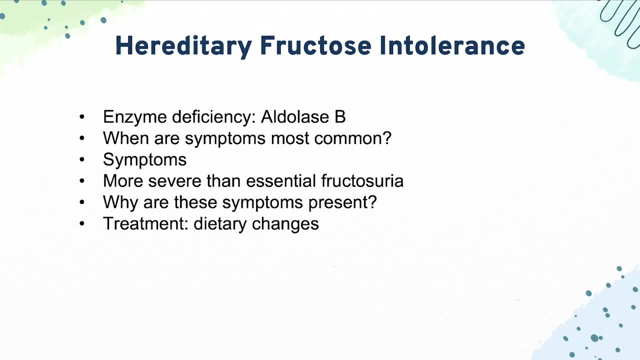 which is essentially the only symptom of essential fructose area And besides that it's a generally benign condition. That's in contrast to hereditary fructose intolerance. So with this condition you have a deficiency of aldolase B, And what aldolase B does is it converts fructose 1-phosphate. 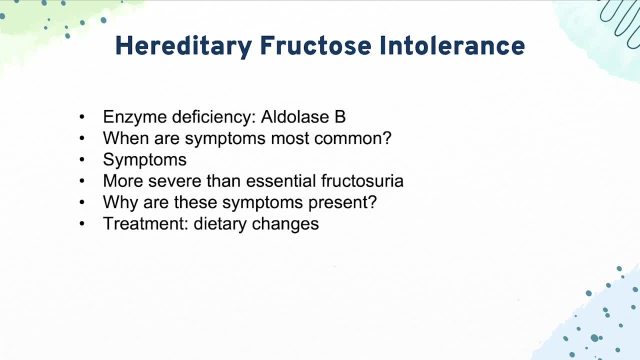 to dihydroxyacetone phosphate, or DHAP, and glyceraldehyde or GAP. So because of that you get an increase in fructose 1-phosphate in the cells. You typically get the symptoms after having things that have fructose. 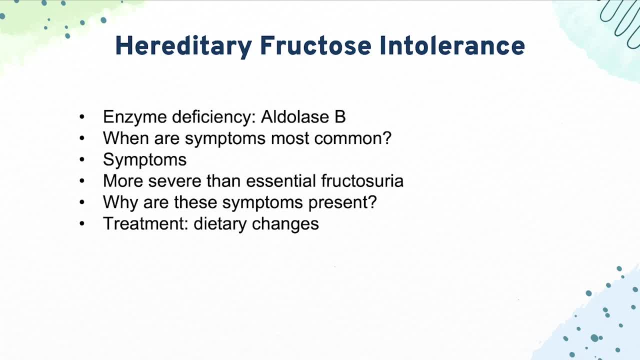 So for instance, any kind of sweet or fruit. So the symptoms and why they're present all ties back into the pathogenesis. So when you have hereditary fructose intolerance and you have trapping of the fructose 1-phosphate inside the cell, 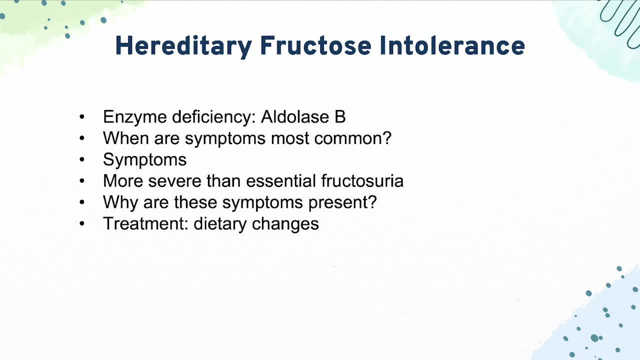 because the phosphate traps it inside the cell. that leads to a lack of available phosphate, because all the phosphate is bound up in the fructose 1-phosphate. Because of that you disrupt glycogenerolysis and gluconeogenesis And because of that you can get symptoms of hypoglycemia, jaundice. 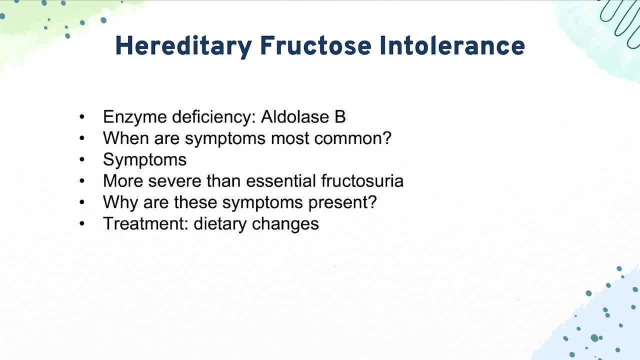 and vomiting. So it is a relatively severe disease and the main treatment for it is just changing things in the diet. So you want to decrease your intake of fructose and molecules that compose fructose, like sucrose, and generally staying away from those foods. 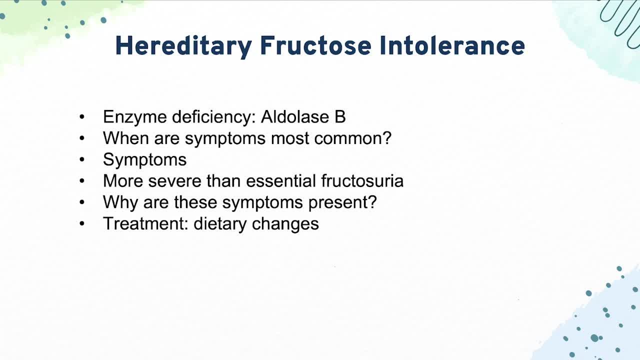 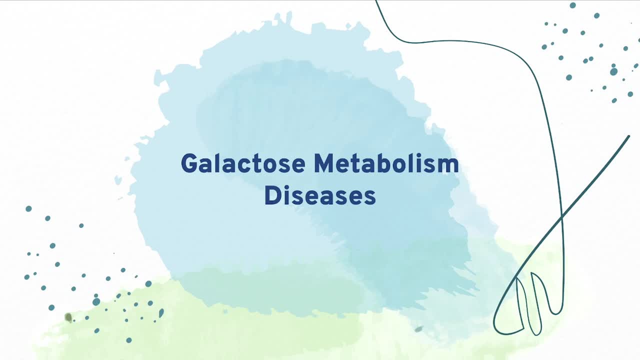 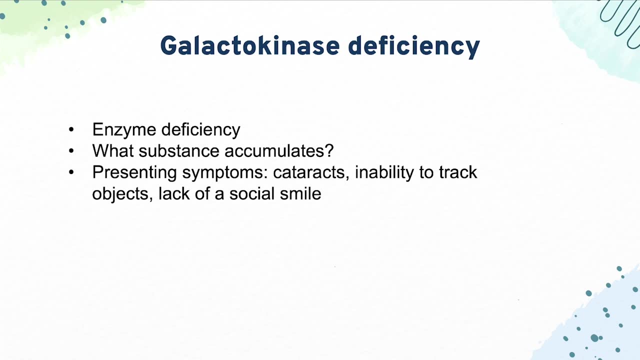 so you don't have the increase of fructose 1-phosphate inside the cells. Our next topic is the galactose metabolism disorders. So with a galactokinase deficiency, this is a little bit similar to essential fructose area, in that you don't have the enzyme required. 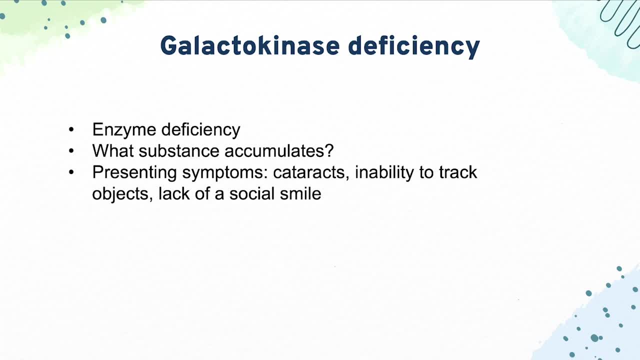 for the phosphorylation of the sugar in question. So here you can't convert galactose to galactose 1-phosphate, So the galactose will accumulate in the blood and urine. As I said before, the galactokinase deficiency. 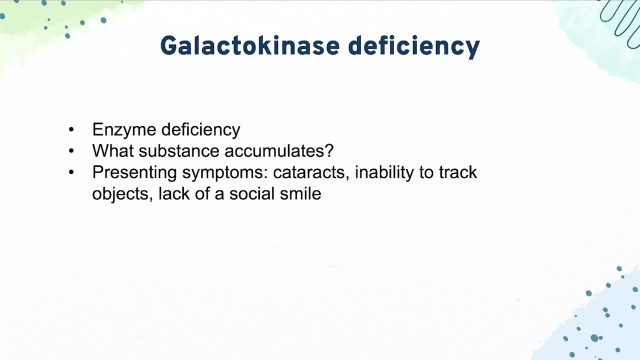 is a bit more severe than the essential fructose area and that just manifests with a couple of actual symptoms. So one of them is cataracts in the eye, another is an inability to track objects and never developing a social smile around others. 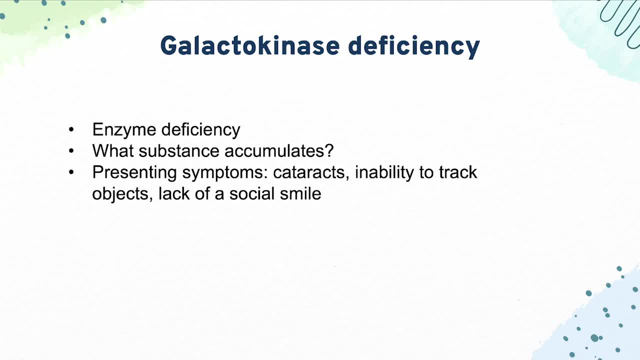 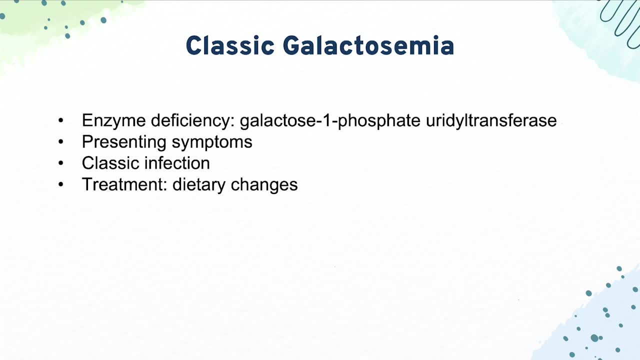 Which is a bit of a weird presentation, but it can be a giveaway on an exam. Then we come to classic galactosemia, which is an enzyme deficiency of galactose 1-phosphate irritable transferase. For the presenting symptoms, 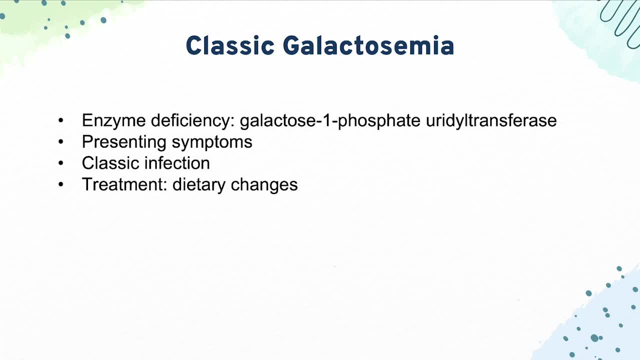 these typically come after the infant has galactose, which is often present in breast milk. So once the baby starts breastfeeding, this can manifest in symptoms. if they have the condition. The symptoms typically involve cataracts, an enlarged liver, jaundice. 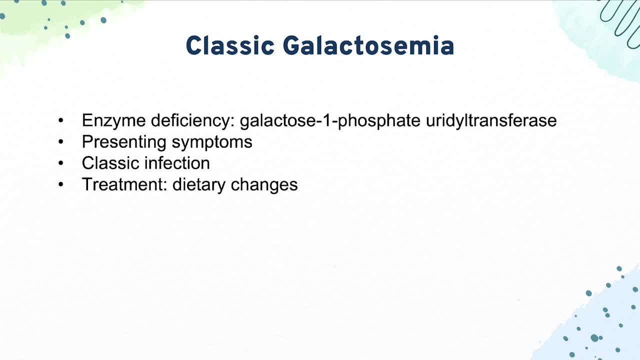 and just overall failure to thrive. One of the commonly tested infections in patients with classic galactosemia is E coli sepsis in neonates, and the treatment, as with hereditary fructose intolerance, is changing your diet, So you want to not have galactose in your diet. 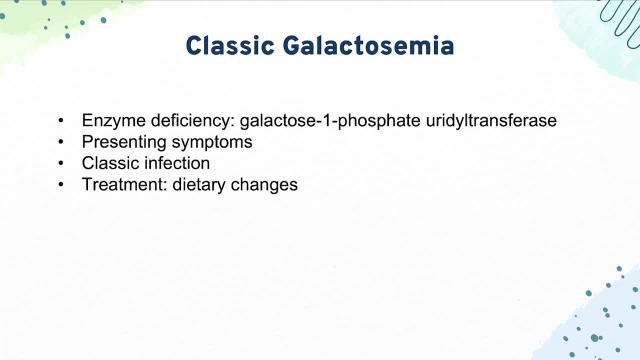 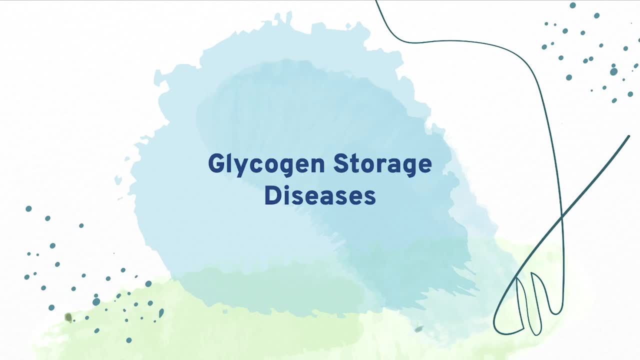 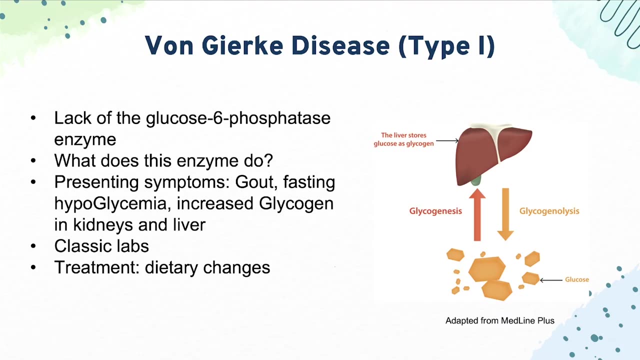 and other things that include galactose, such as lactose. Next we come to the glycogen storage diseases, which are all very high yield, and you are essentially guaranteed to have a question on one of these. Our first one is von Gierke disease, or type 1.. 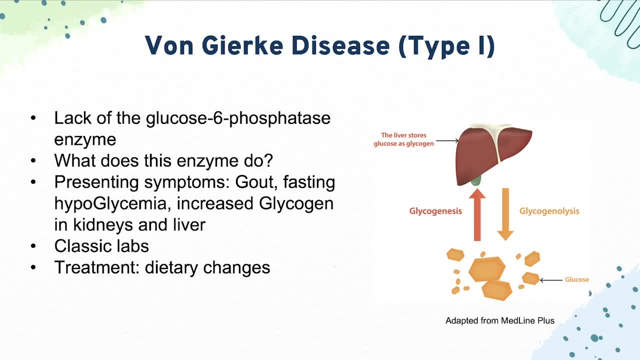 The enzyme that's deficient is the glucose 6-phosphatase enzyme. So glucose 6-phosphatase is going to remove, as phosphatases do remove, the phosphate from the molecule, And without the phosphatase you are left with G6P, just kind of stuck there. 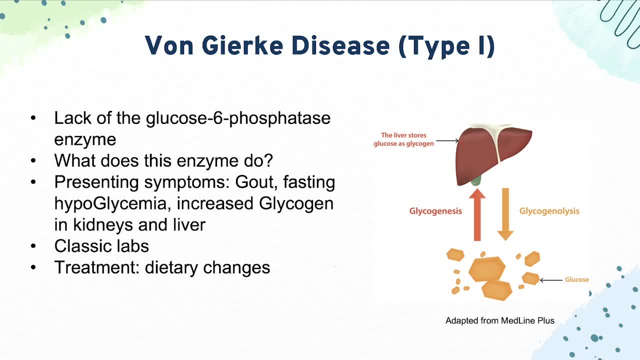 because you can't remove the phosphate. The presenting symptoms can be remembered because they all have a G in them. So things like gout, fasting, hypoglycemia and increased glycogen in the kidneys and liver For the classic labs. 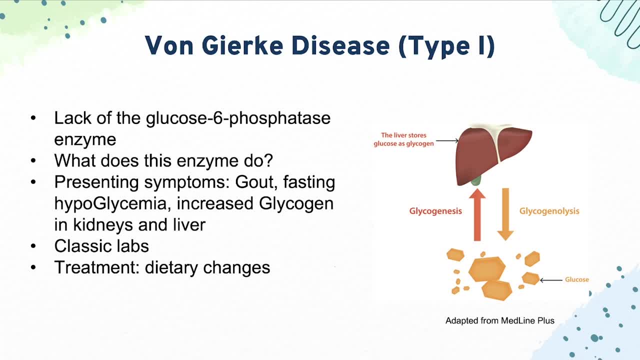 you also can get elevated urate levels, elevated triglycerides and elevated blood lactate levels, So that entire picture on a step exam, step exam, stem would probably clue you into von Gierke disease. The treatment as before. 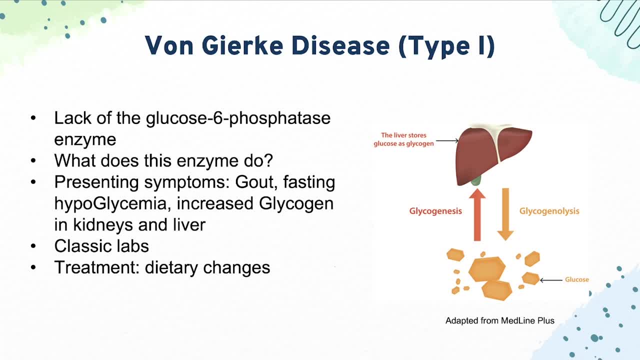 you're probably seeing a theme by now is dietary changes. So what you want to do is avoid certain sugars that can lead to exacerbations of the condition. So you want to give cornstarch orally as often as you can, because by giving that 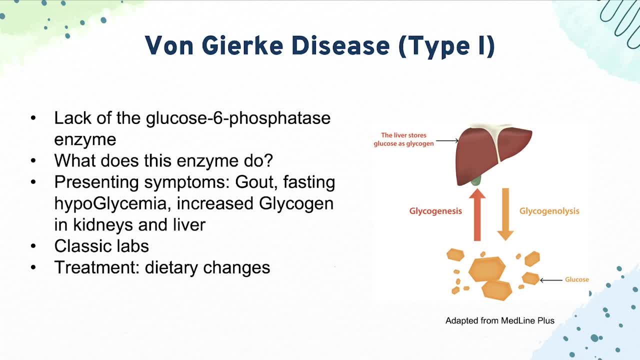 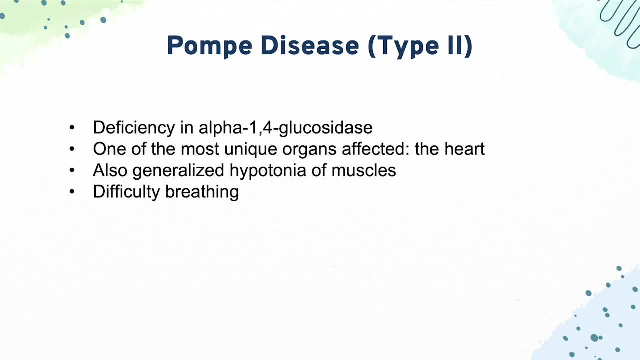 you can keep the gluconeogenesis and glycogenolysis going For Pompe disease, which is type 2, that's a deficiency in alpha 1,4-glucosidase, And one of the most unique organs affected in this condition is the heart. 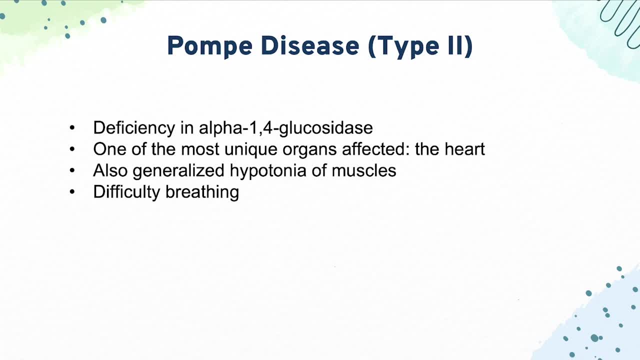 So if they mention that the patient is young and has maybe a cardiomyopathy and can't really tolerate any sort of exercise, that can be indicative of Pompe disease. Also, they can present with generalized hypotonia of the muscles, so low tone. 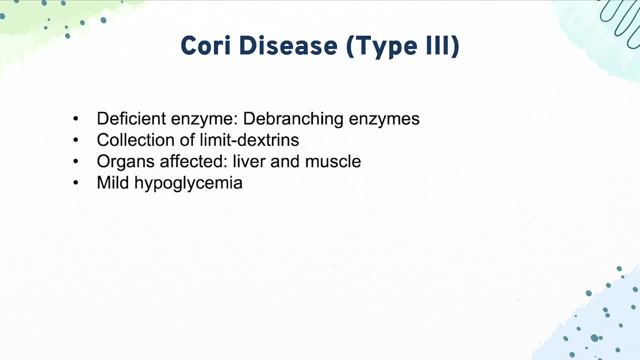 and overall difficulty breathing. Cori disease is type 3, and it's similar to the von Gierke disease- type 1, but it's a bit not as severe. So, unlike in von Gierke disease, here you have normal blood lactate levels. 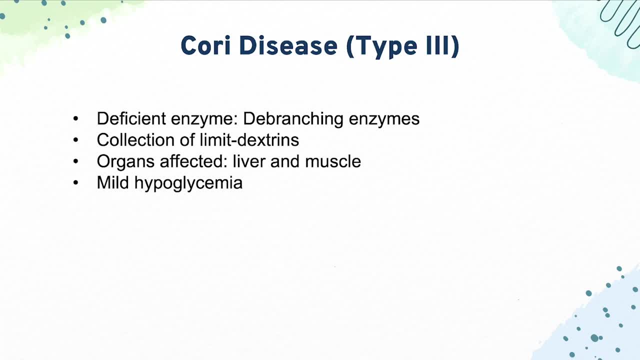 And your deficient enzyme is the debranching enzymes, which remove bits of glucose from glycogen. When you have a deficiency of the debranching enzymes, you are left with a collection of these things called limit dextrins in the cells, The organs that are primarily affected. 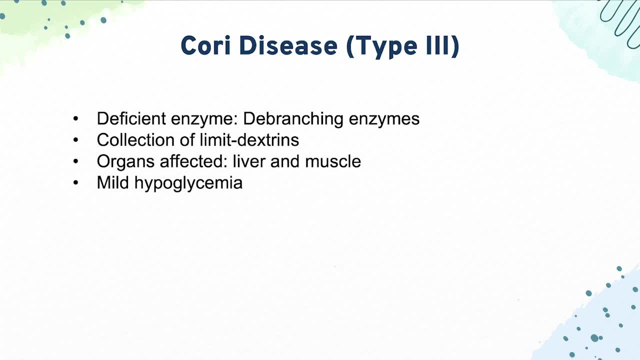 are the liver and the muscle and it can lead to a mild hypoglycemia because you are impairing the process of glycogenolysis In Cori disease. you aren't affecting gluconeogenesis because this condition only affects the debranching enzymes. 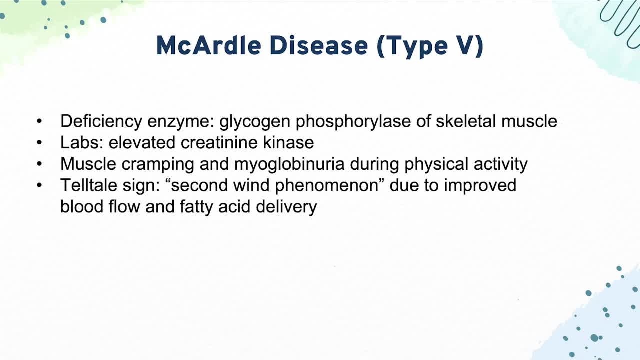 Our next one is McArdle disease, which is also called type 5.. The deficient enzyme is glycogen phosphorylase, primarily in skeletal muscle, And for your labs you're going to have an elevated creatinine kinase For your symptoms. 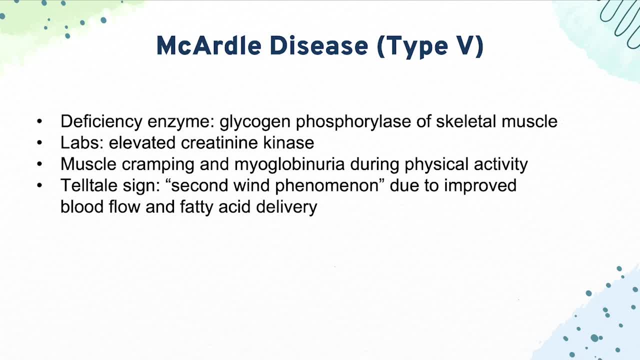 you're going to have muscle cramping and myoglobinuria during physical activity. But one of the main signs that can kind of give this away on an exam is something called the second wind phenomenon. So with that you have exhaustion after exercise, but then you get a second wind. 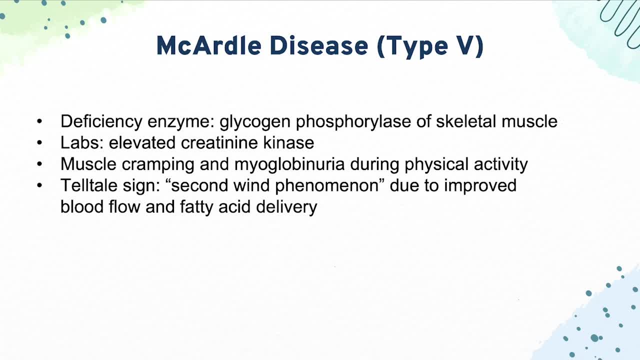 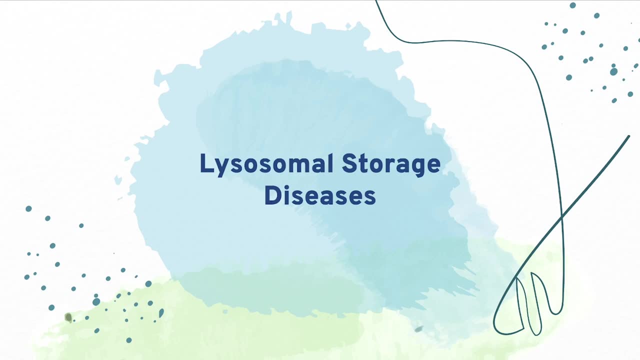 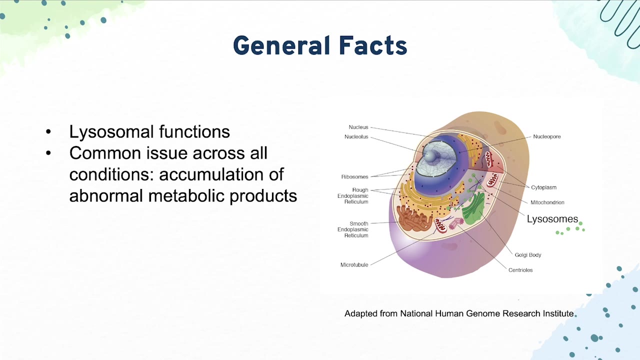 And that's because of improved blood flow and fatty acid delivery And all of those things together kind of give a picture of McArdle disease. Our next topic is lysosomal storage diseases. So some general facts about the lysosomes. They are essentially the cell's trashcan. 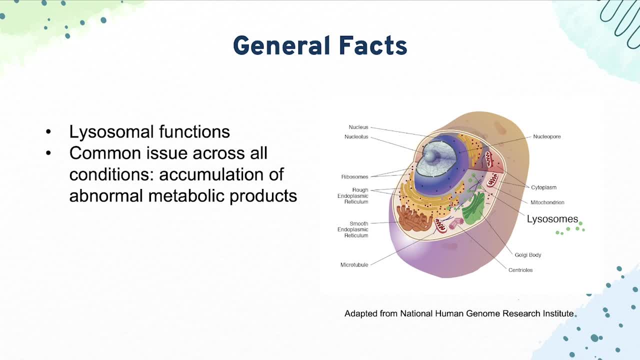 They function at a low pH, So they're acidic, and they use a collection of digested enzymes, So like proteases and lipases, to digest molecules that are no longer needed in the cells. When you have an issue, then, with the lysosomes. 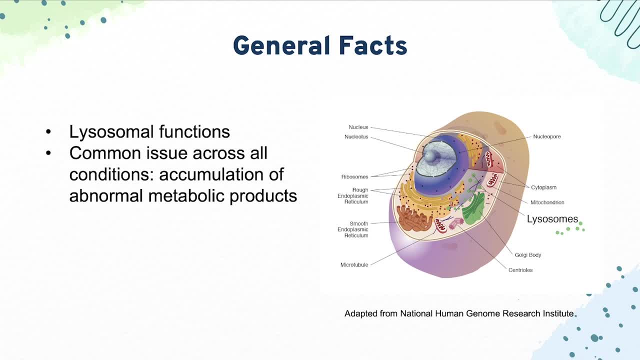 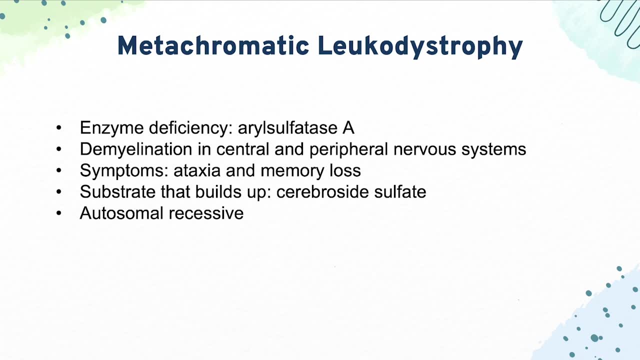 you get an accumulation of those abnormal metabolic products which can lead to issues. So our first condition is metachromatic leukodystrophy. The enzyme deficiency in this case is aerosulfatase A, And it's primarily characterized by demyelination. 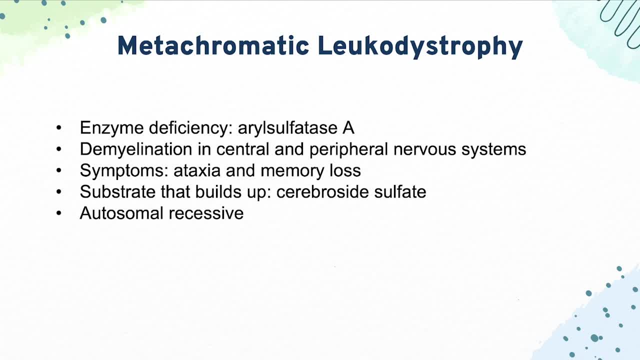 in the central and peripheral nervous systems And overall that leads to things like ataxia, memory loss and dementia. The substrate that builds up, because aerosulfatase A is deficient, is cerebroside sulfate, And it's good to keep in mind. 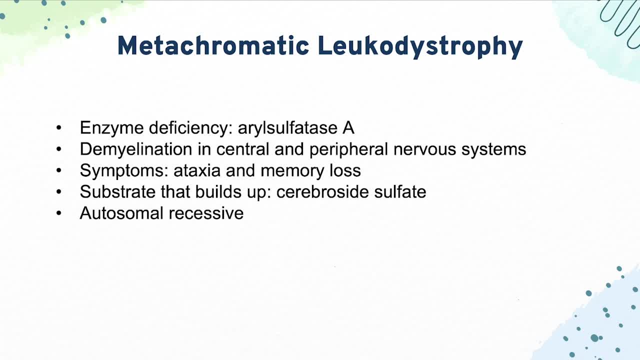 the inheritance pattern for all these diseases. So this one is autosomal recessive. That's the case for most of them. If you happen to forget on the exam which condition is which inheritance pattern, I would go with autosomal recessive, unless you are confident. 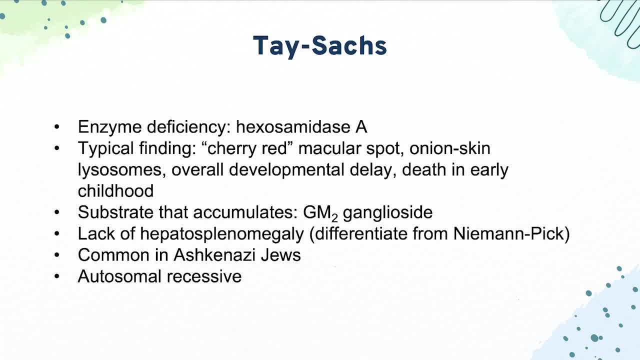 of the ones that differ, which we'll get to in a bit. Our next one is Tay-Sachs. So here you have a deficiency of hexosamadase A, And the typical finding is a red spot on the macula, called a cherry red macula. 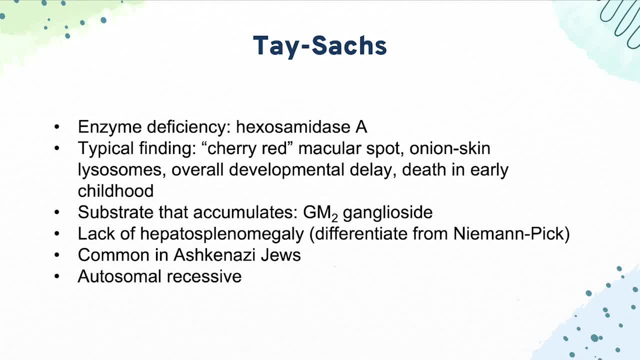 You also can see onion skin lysosomes on pathology And other symptoms are just developmental delay and otherwise death in early childhood. The substrate that accumulates because you are deficient in the hexosamadase A is the GM2 ganglioside. 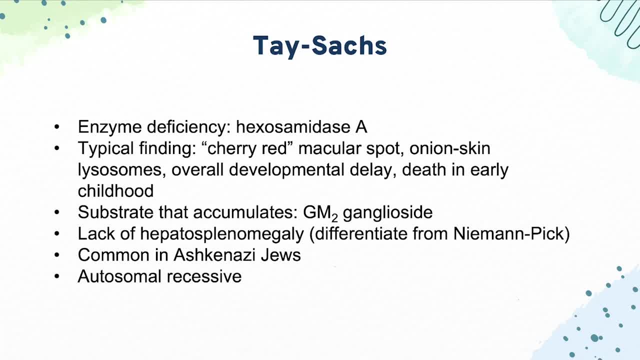 And one of the things to know about Tay-Sachs is how to differentiate it from another disease which we'll get to soon, called Niemann-Pick, Because they do present very similarly. Tay-Sachs has the ability as a lack of hepatosplenomegaly. 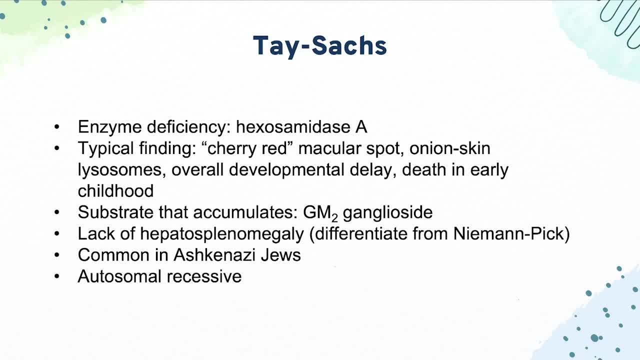 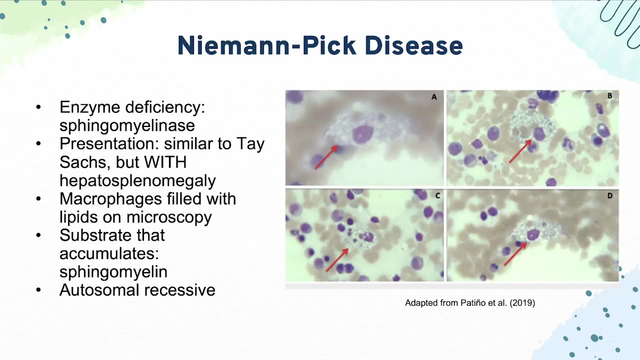 So you're going to have a normal sized liver and spleen in this case. Tay-Sachs is pretty common, or relatively common, in Ashkenazi Jews And it is autosomal recessive Niemann-Pick disease. So the enzyme deficiency here. 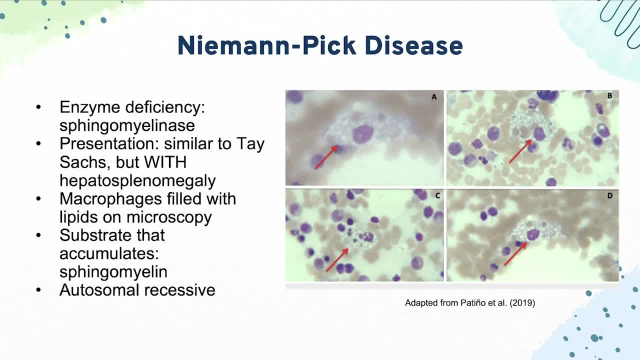 is stingomyelinase And that leads to an accumulation of stingomyelin. As I was saying before, the presentation can be very similar to Tay-Sachs. You even have that same cherry red macula, But here you do have hepatosplenomegaly. 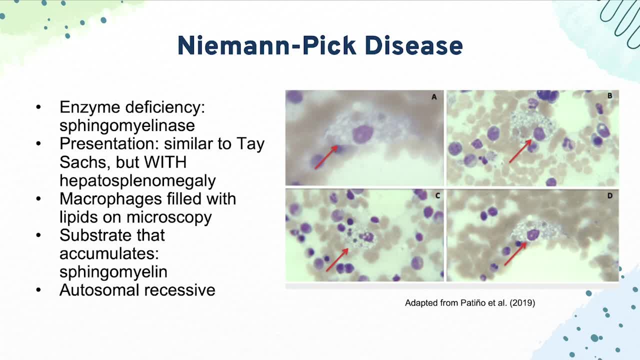 If you were to look at some of the macrophages and just cells under microscopy, you would see that they have lipids. Those can be called foam cells And the inheritance pattern is autosomal, recessive. Fabry disease, The enzyme deficiency. 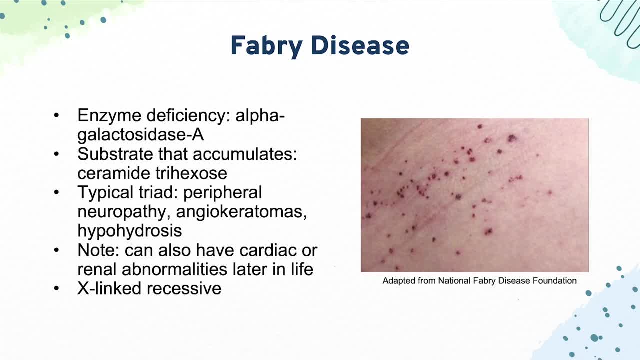 is alpha-galactosidase A. The substrate that accumulates because of the enzyme deficiency is ceramide trihexose, And here you have a typical triad. you're going to want to commit to memory, So you're going to have 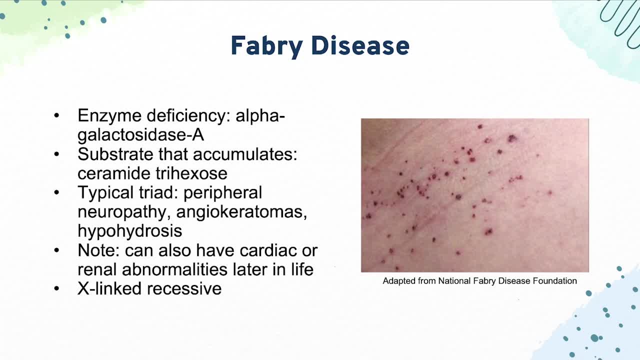 peripheral neuropathy, So just general tingling and numbness in your hands and feet, Angiocaritomas, which you can see an example of on the screen on the right. I would know that picture in case they test an image of it. 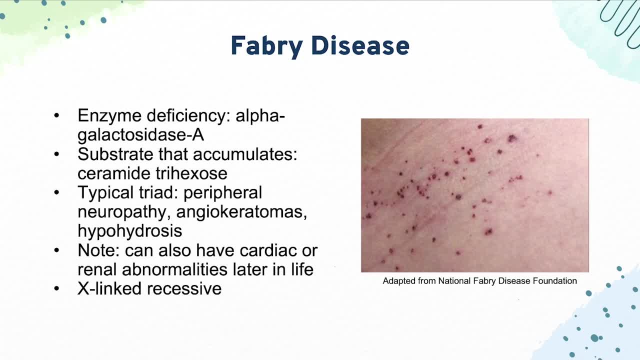 And hypohidrosis, So just an inability to sweat or just an impairment of overall sweating. Patients with Fabry disease can have kidney or heart issues later in life And this is one of the conditions that deviates from the norm of things, being autosomal recessive. 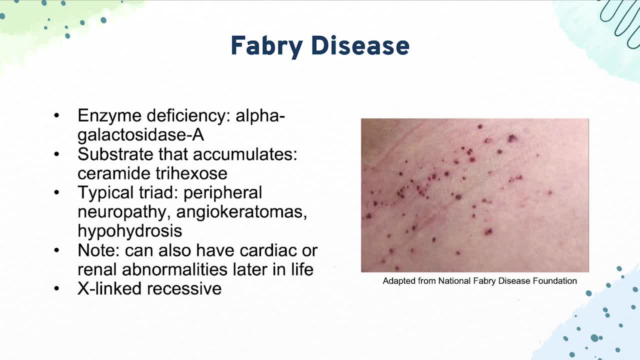 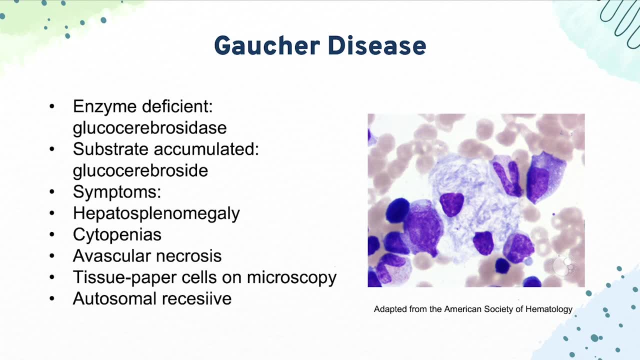 Here it is added. Here it is excellent- recessive. Next we have Gaucher disease and the enzyme deficient is glucocerebrosidase. The substrate that's accumulated is glucocerebroside And these symptoms are a bit different from others. 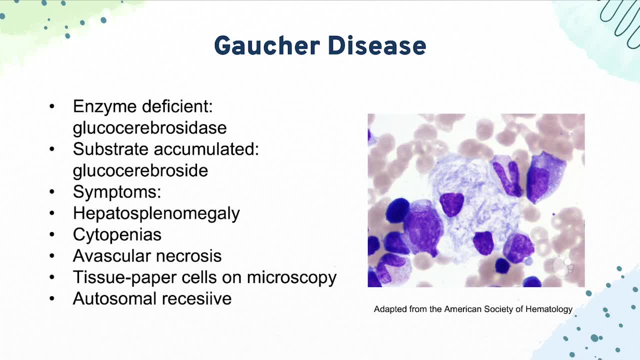 which makes it a bit easier to spot. So you have hepatophilomegaly, which is nonspecific, But you also have cytopenias, So a lack in one or many blood cell lines And avascular necrosis, often of the femur. 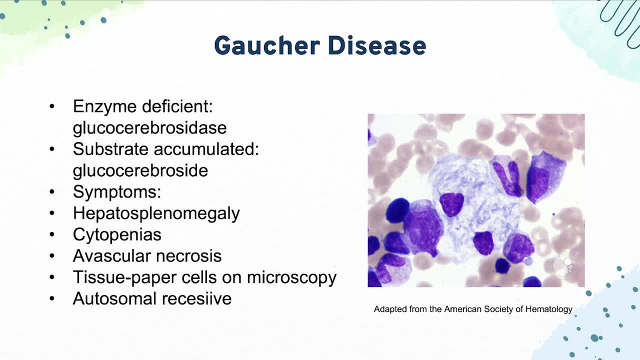 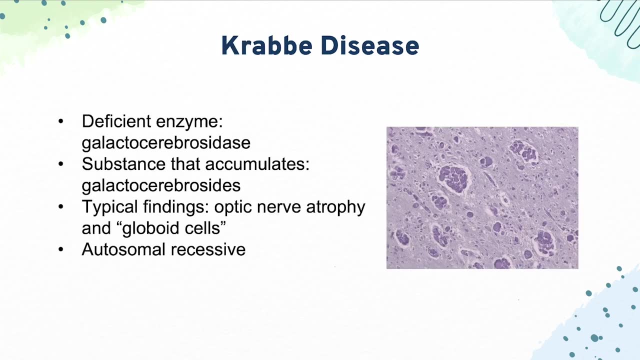 If you have tissue paper cells on microscopy, as shown to the right, that can be also indicative of Gaucher disease And it is autosomal recessive, as many of the other conditions are. Next we have Krabbe disease and the deficient enzyme is galactose. 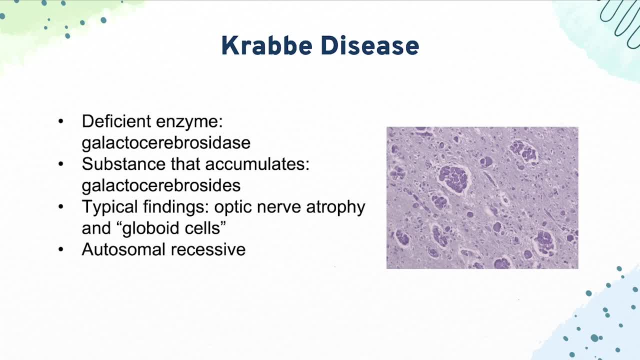 Galactoserebrosidase. So this does sound similar to the enzyme deficient in Gaucher disease called glucocerebrosidase. So just make sure that you don't confuse them. The substance that accumulates is galactoserebrosides. 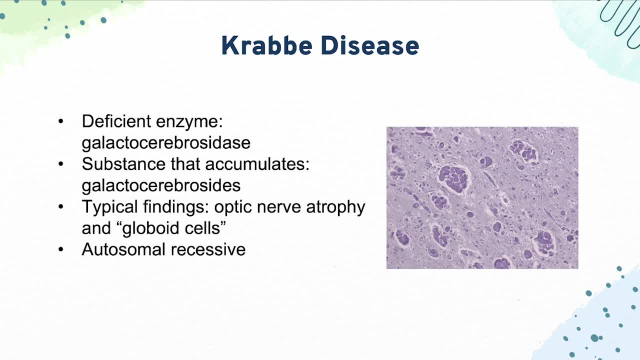 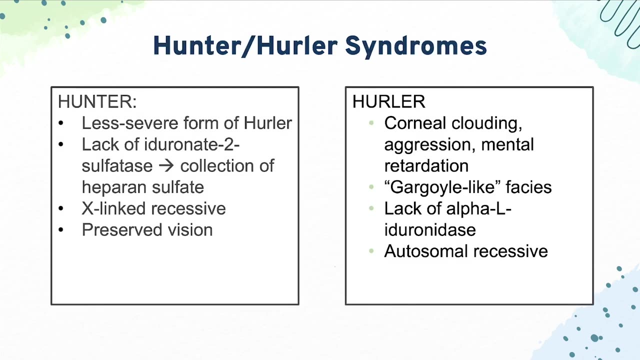 And the typical findings are optic nerve atrophy, so eventual blindness, and globoid cells which you can see on the right. Like the many of the other conditions, it is autosomal recessive. Next we come to Hunter and Hurler syndromes. 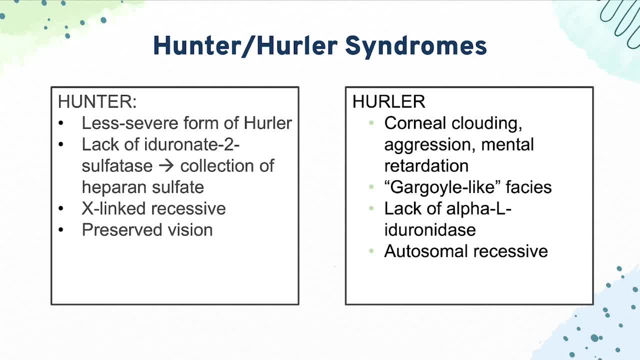 These are called the mucopolysaccharidoses And they have some commonalities, but they're also a little bit different. So let's start with Hunter disease. So it's a bit less severe than Hurler disease And it's a lack of the enzyme. 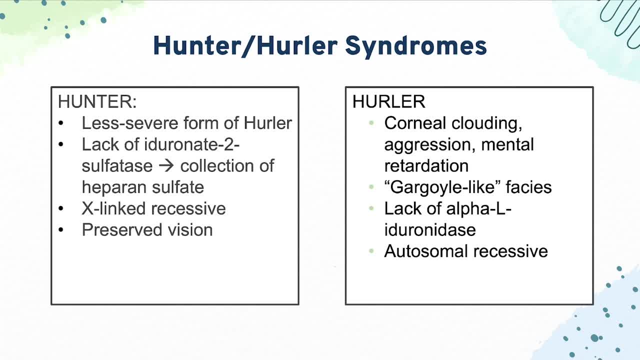 iduronate to saltine. It has a lot of ribosulfatase which leads to a collection of heparin sulfate. It is X-linked recessive. That's the other X-linked recessive disease besides Fabry disease. And here you have. 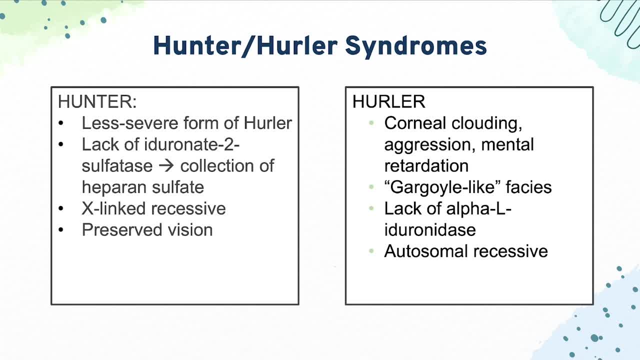 preserved vision. That's in contrast to Hurler disease, where you have. One of the common findings on a physical exam is gargoyle-like phase Cs as well, And here it's a lack of alpha-L-iduronidase. So the enzymes sound similar, but they will often put both of those enzymes in the potential. 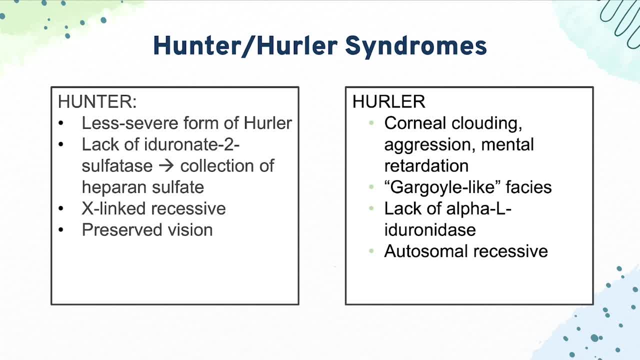 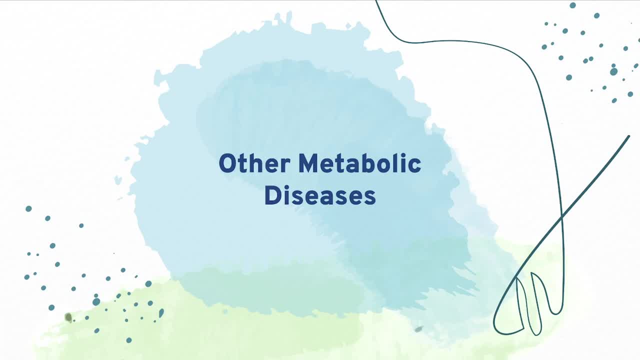 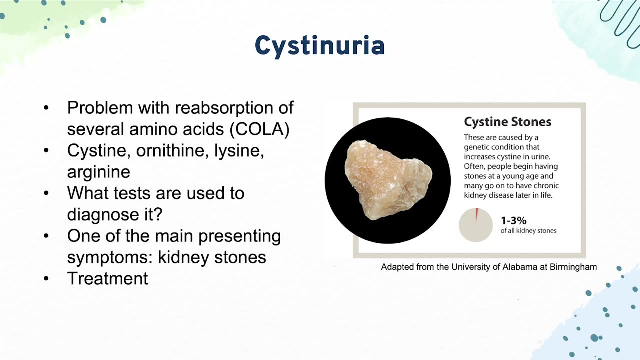 answer choices. So make sure you can differentiate the two. And it is odds a little more excessive, Some other metabolic diseases. So our first one is cystinuria. Here you get a defect with reabsorption of a couple of key amino acids. 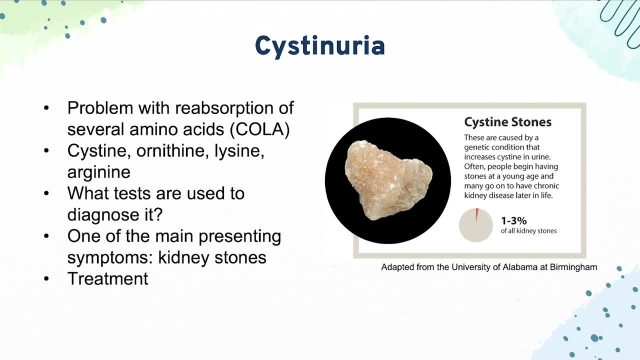 These are cysteine, ornithine, lysine and arginine. They're called together the cola amino acids just because of the first letters of each name And the tests used to diagnose it. Um, primarily is the sodium cyanide nitropresside test. 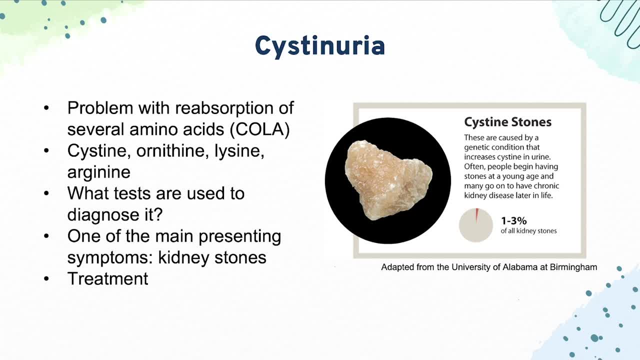 Um, one of the main symptoms that it presents with is kidney stones, because when you don't reabsorb these enzymes, they can precipitate out in the urine and obstruct the flow of urine. And, as a quick review um you would see hexagonal cysteine stones on microscopy. 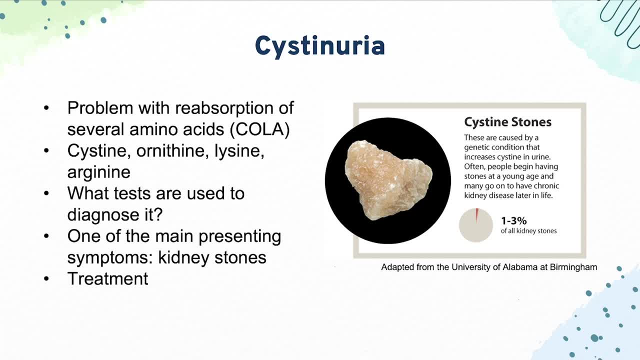 The treatment for cystinuria Is um alkalinizing the urine, making it more basic with things like potassium citrate. That's going to help make the amino acids more soluble, because when you make the urine more alkaline, the acids can dissolve in it more easily. 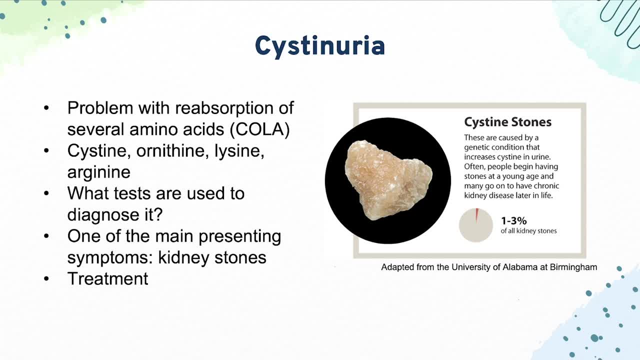 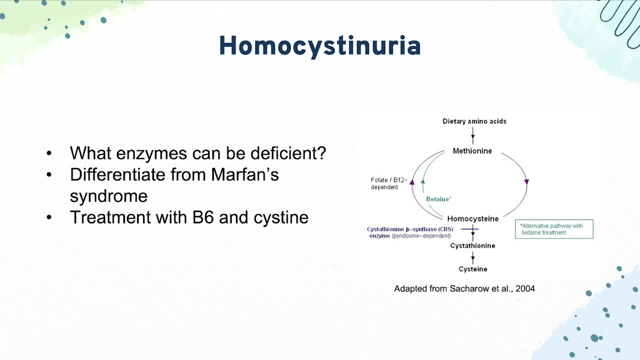 And you also want to have a diet low in methionine and you also want to just generally hydrate. well, Now we have homocystinuria, Um, and here you can have two main deficient enzymes. So one of them is cystathionine beta synthase. 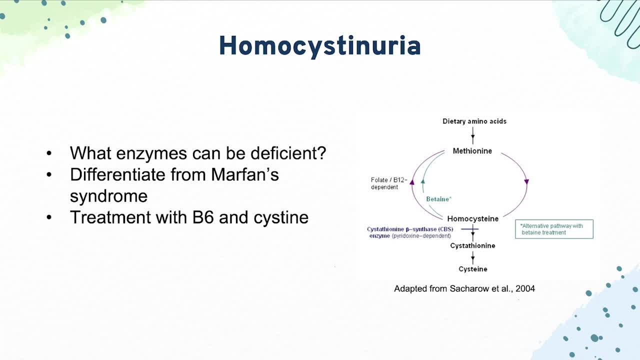 The other is methionine synthase, So that can lead to a collection of different sort of substrates. If you don't have the methionine synthase, you get an increase in homocysteine, And if you don't have cystathionine synthase, you also get an increase in homocysteine. 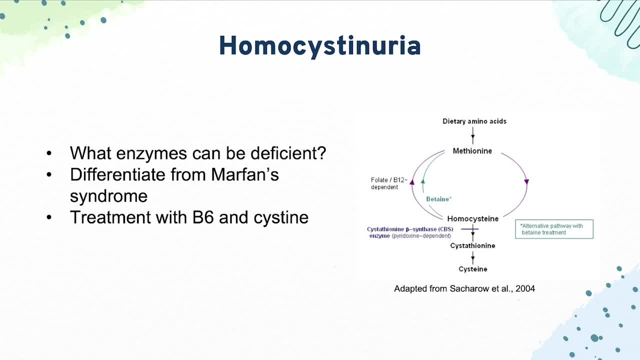 And if you don't have the methionine synthase you also get an increase in homocysteine levels. Marfan syndrome can be a bit similar to homocystinuria, because in both conditions they have the Marfanoid habitus. 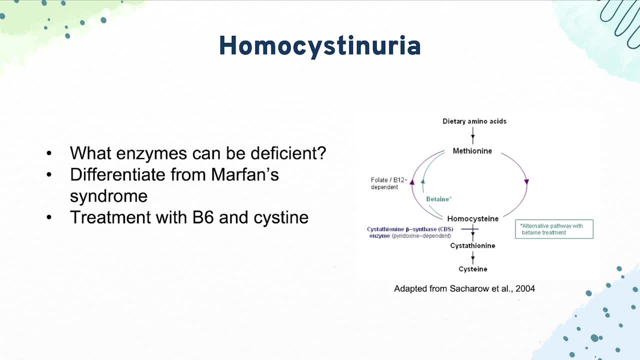 They can have lens dislocation and cardiovascular effects. The main difference for homocystinuria- that's good to know- is that you have the lens dislocating in a different direction. So in Marfan disease the typical lens dislocation is up and out. 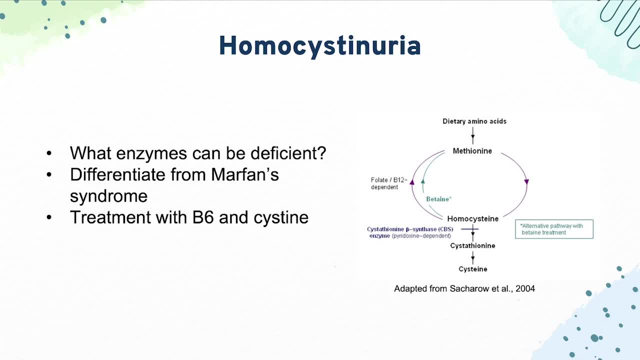 It's supralateral. for homocystinuria, The lens dislocation is inframedial, So it's down and in and that's one of the typical ways they try to get students to tell apart those two conditions. Um, the treatment is with B6 and cysteine. 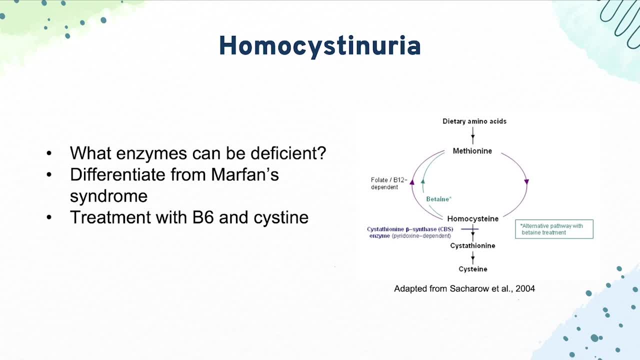 So if you have B6, that can strengthen the function of the endometrium. So if you have B6, that can strengthen the function of the endometrium. So if you have B6, that can strengthen the function of the endometrium. 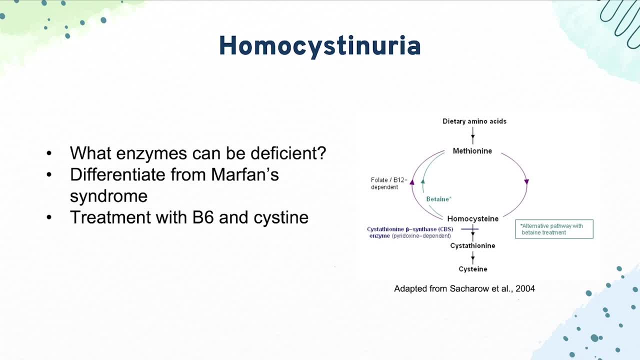 The enzyme cysteine synthase because it uses B6 as a cofactor. As you can see on the screen, it's pyridoxine dependent For treating with cysteine. it just supplies the downstream sort of substrate that's lacking. 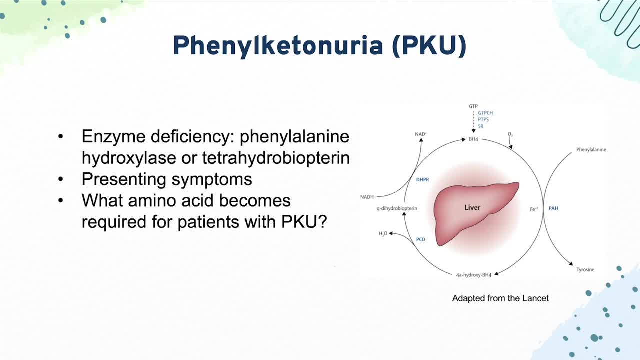 Then we come to phenylketonuria, which is a deficiency of one of two enzymes. So the first enzyme is phenylalanine hydroxylase, The second is tetrahydrobiopterin. So there are typical symptoms that present with PKU. 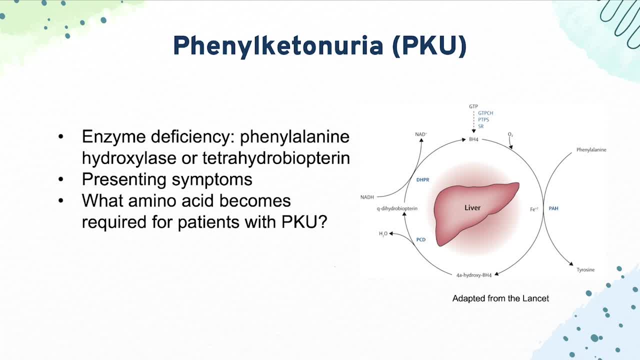 One of the common ones is skin that is hypopigmented. You also can have a weird off-putting musty body odor and overall intellectual disability, And one of the things that's good to know for PKU is that tyrosine becomes essential as an external cofactor. 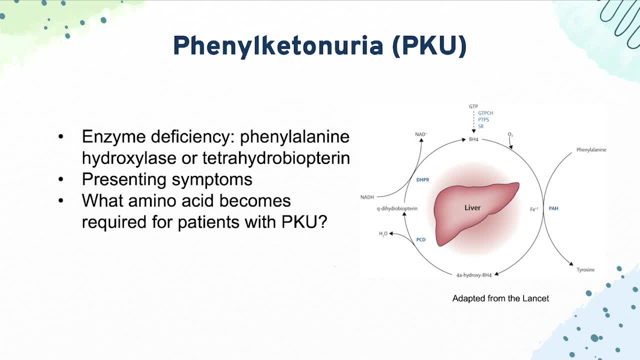 Because phenylalanine is used to make tyrosine. if you don't have the enzyme that converts phenylalanine into tyrosine, you have to get it from somewhere else, So the treatment becomes to supply with tyrosine. 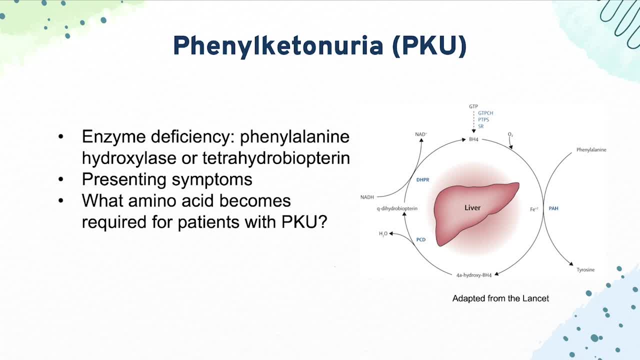 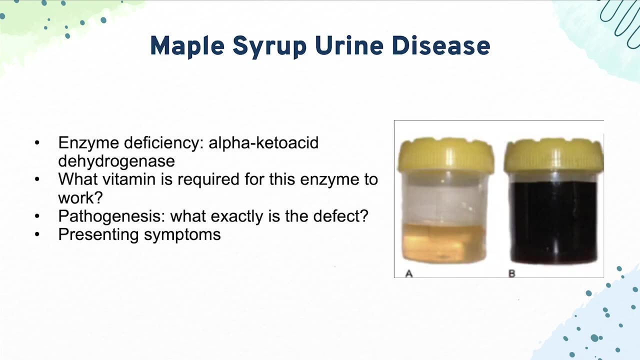 The other treatment in general is just to avoid foods that have phenylalanine. They make specialized foods on the market for these patients, And patients should usually subsist on those to avoid flare-ups of their disease. Next we come to maple syrup urine disease, which is so named because of how the disease presents. 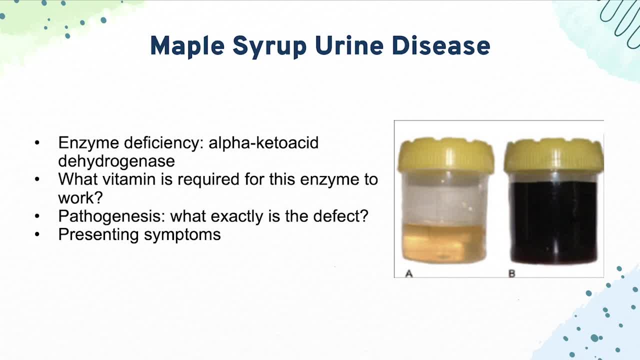 The urine tends to look like maple syrup, as you can see on the right. The enzyme deficiency is alpha-ketoacid dehydrogenase, which, as a pearl, requires thiamine or vitamin B1. B1 is needed for a lot of dehydrogenase activity. 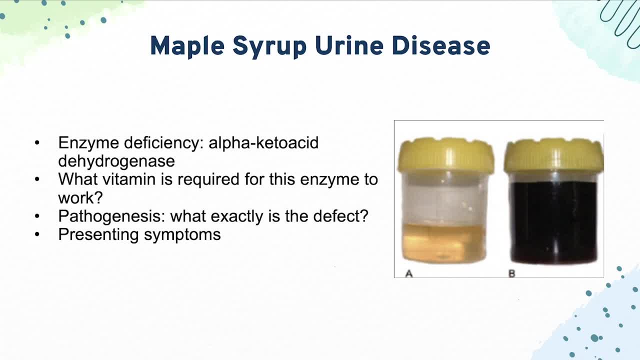 So if you see dehydrogenase and they ask which vitamin is needed to supply that sort of enzyme, go with B1. The defect is that you can't break down branched amino acids, so things like valine and isoleucine. 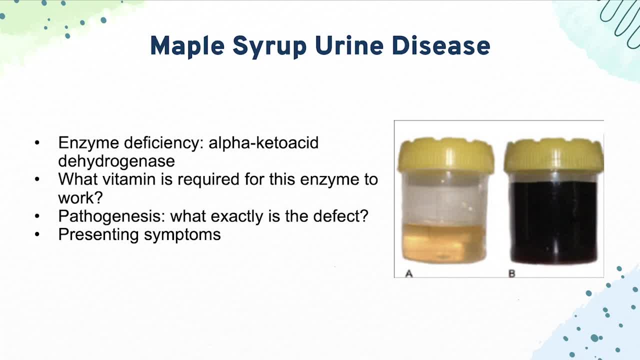 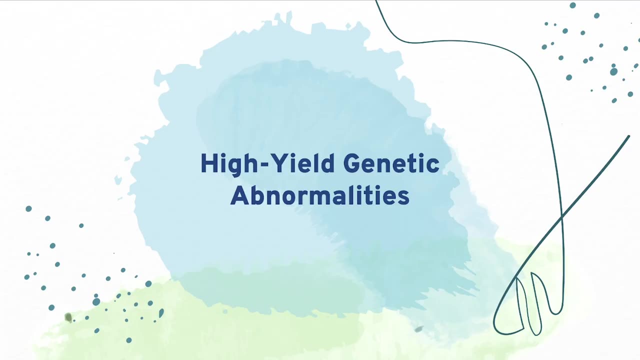 So those will accumulate in the blood. The symptoms are, besides the presence of the dark brown urine, you just get things like vomiting and poor feeding. Next we come to the high-yield genetic abnormalities, and this is actually our last topic. 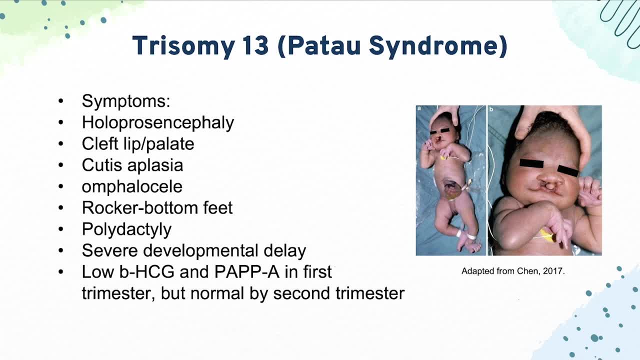 So trisomy 13 is tau syndrome. As a quick review, a trisomy is three copies of one chromosome. So in the human body, or the regular human body, there are 46 chromosomes per cell and you have two copies of each. 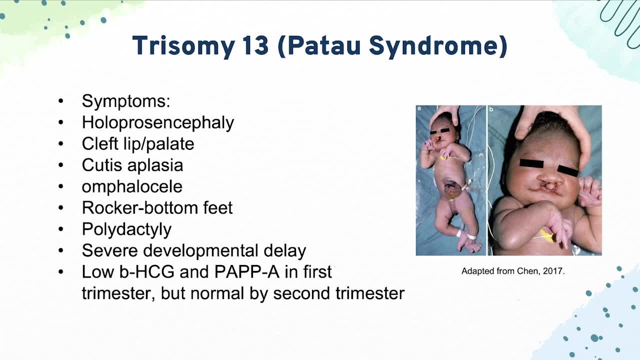 So two of chromosome 1,, two of chromosome 2, and so on. And then you also have the sect chromosomes, which would be XX or XY. With trisomy 13,. instead of having two copies of the 13th chromosome, you'd have three. 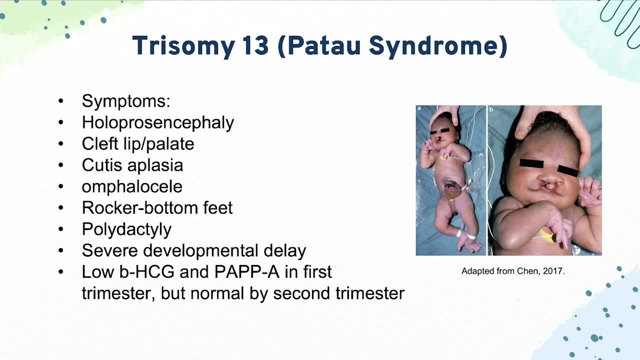 So the symptoms are holopresencephaly, a cleft lip and palate cutis, aplasia, which is kind of marked by a defect in the calvarium. You also can have an omphalocele in the abdomen, rock or bottom feet, polydactyly, a severe developmental delay. 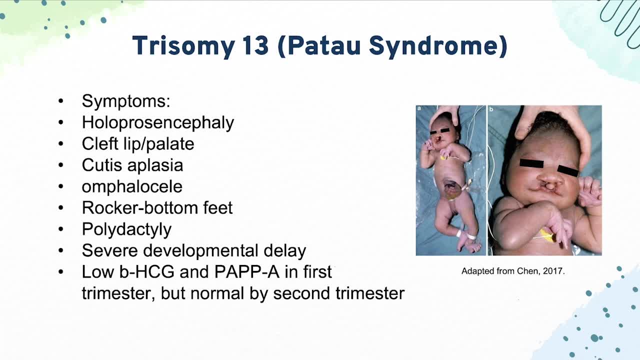 And for the labs which can be used to predict this. you could have a low beta HCG And PAPPA in the first trimester But, of note, these do normalize by the second trimester And the prognosis for this condition is usually very poor. 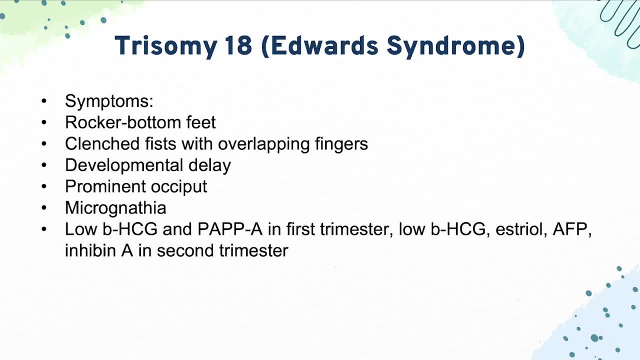 Children often die in the first year, unfortunately. Our next condition is trisomy 18, or Edwards syndrome, And the high-yield symptoms for this are rock or bottom feet, clenched fists with overlapping fingers. that's a main one. 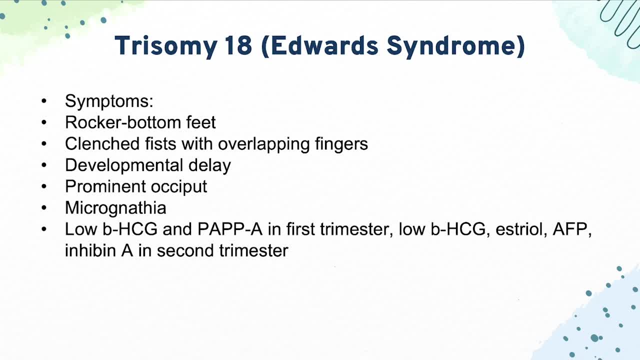 development, mental delay or intellectual disability, a prominent occiput or back of the head, micrognathia. And for your labs you would have a low beta HCG and PAPPA in the first trimester And then in the second you would have low beta HCG, estriol, AFP and inhibin A. 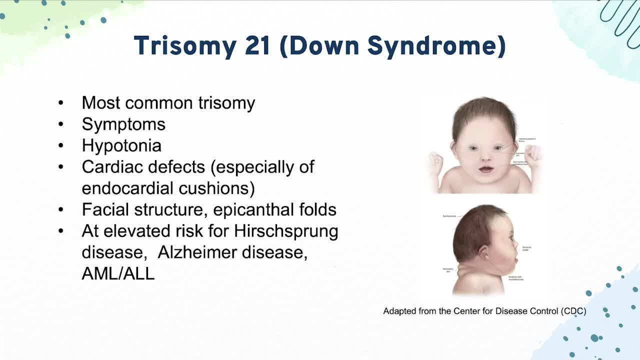 So essentially everything is low. Our last condition is trisomy 21,, or down syndrome. It's the most common trisomy And, unlike trisomy 13 and 18, people can live for long lives with trisomy 21.. 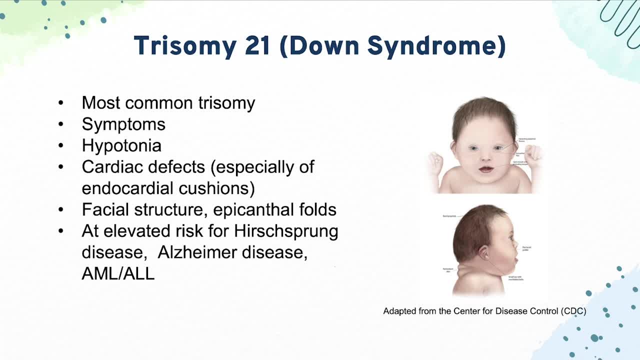 The symptoms are hypotonia, cardiac defects, especially of the endocardial cushions. That can lead to things like a complete atrioceptal defect, And one of the commonly tested things is a change in the facial structure. So you have epicanthal folds, a protruding tongue, upslanting palpebral fissures and things like that. 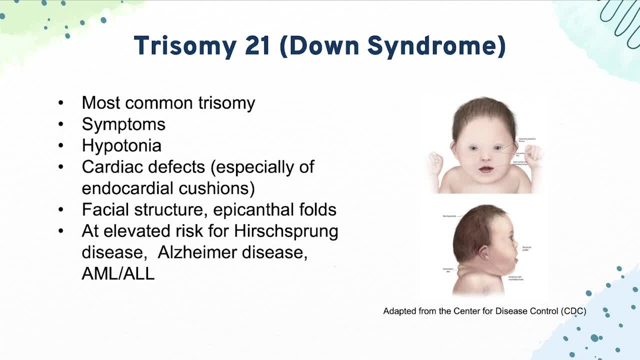 And lastly, these patients are at elevated risk of things like Hirschsprung disease, Alzheimer's disease. That's because the amyloid protein is coded for on chromosome 21.. So if you have an extra chromosome, you have even more of that protein.